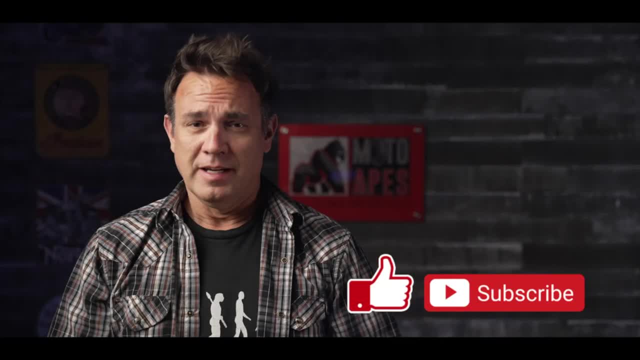 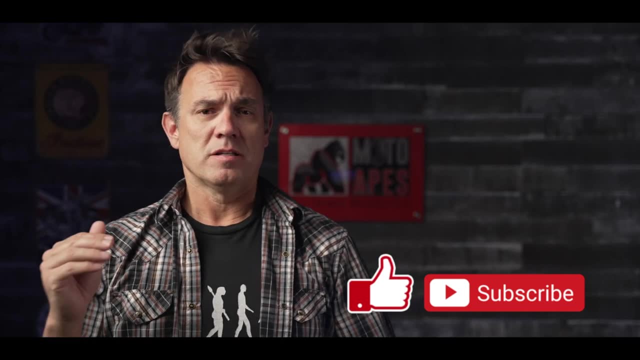 dad used to characterize us as organ donors. It doesn't take an idiot to see motorcycles have two less wheels and aren't wrapped in a cage of metal crossbars and airbags. like cars Smash into anything and it's likely to hurt a whole lot more Riding a motorcycle takes a different set of skills than driving a car, and motorcyclists are more vulnerable to the hazards posed by weather and road conditions. But the question of how safe are motorcycles is a little broad and subjective. Compared to what are motorcycles safer or more unsafe, then? 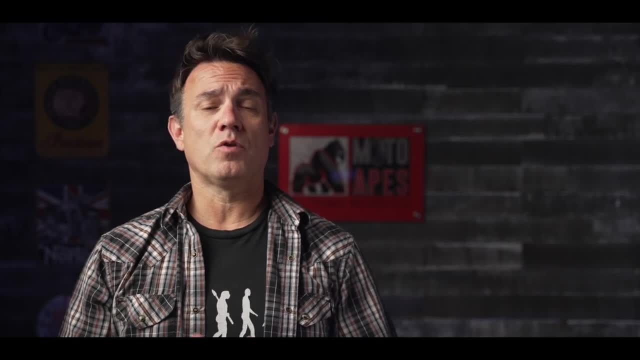 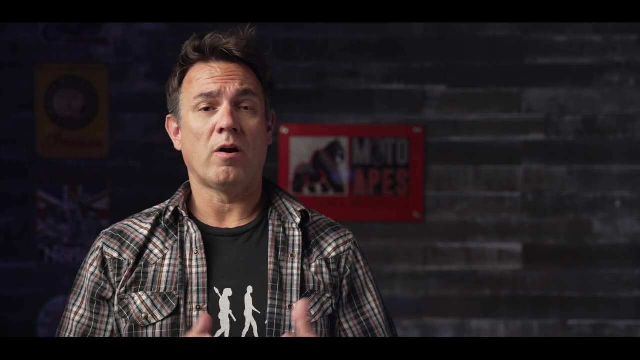 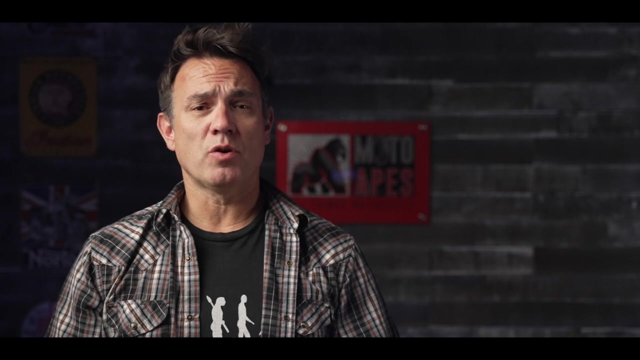 The go-to assumption must be other vehicles occupying the same roadways that motorcycles. But under what conditions and according to what type of rider? where and exactly how do the available statistics prove that motorcycles are unsafe? Anyone digging into the statistics of motorcycle safety will run into some stumbling blocks. Firstly, is the available data From one? 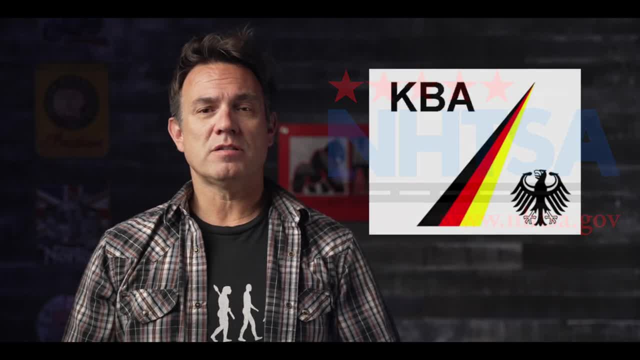 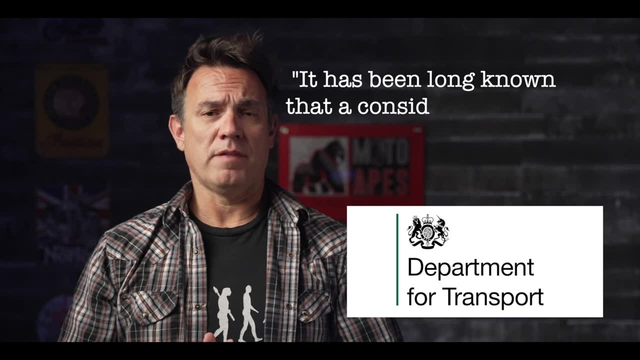 country to the next. the methodology for collecting the data ranges from precise to adjusted, with the Department of Transport in the UK noting that quote. it has been long known that a considerable percentage of non-motorcyclists are more likely to have a death wish than other vehicles. 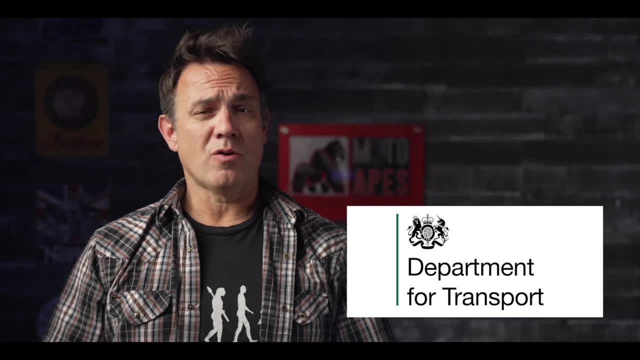 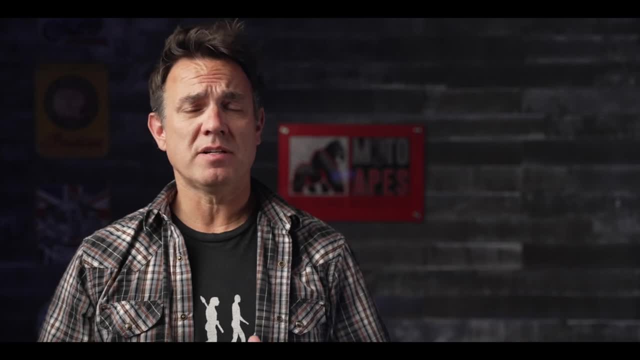 Second, the methodology for collecting the data is that the number of non-fatal casualties are not reported to the police, And how quote? this should be borne in mind when analyzing and interpreting the data. Now, even the National Highway Transportation Safety Administration says the challenge faced when researching motorcycle accidents is the absence of data. 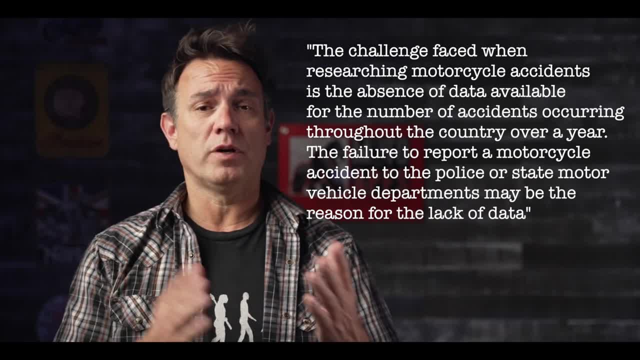 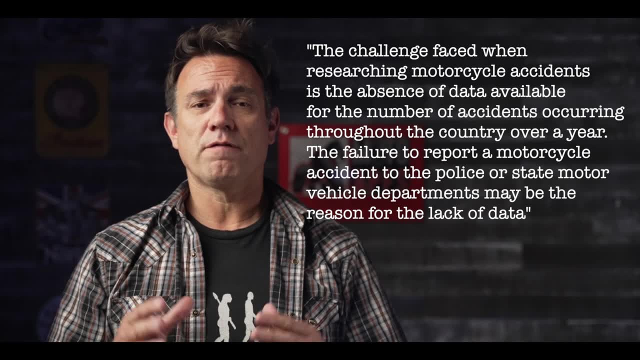 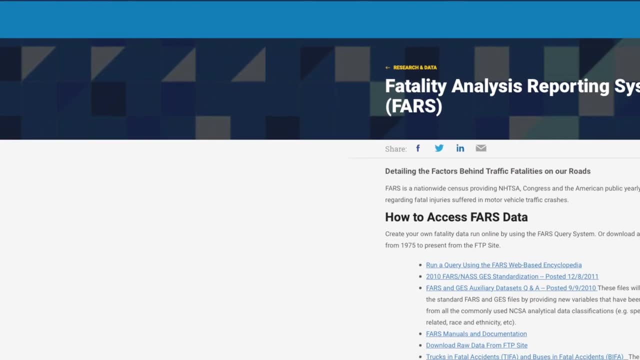 available for the number of accidents occurring throughout the country over a year. The failure to report a motorcycle accident to the police or state motor vehicle departments may be the reason for the lack of data. Furthermore, data in the NHTSA's fatality analysis reporting system, or FARS, include a census of motorcyclist fatalities. 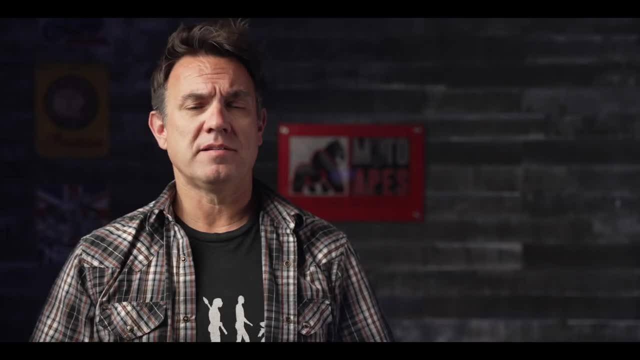 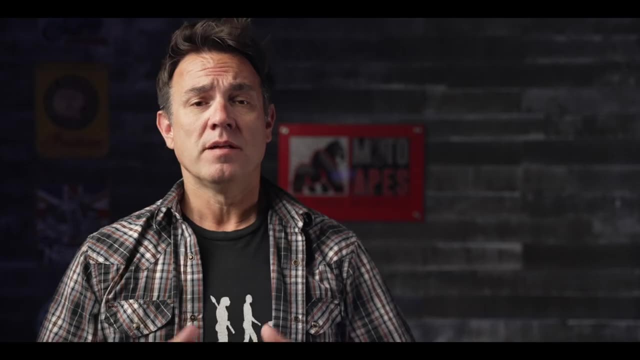 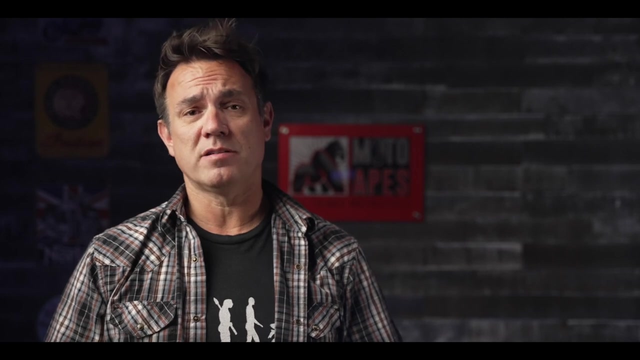 but provide no data on injuries. The NHTSA's National Automotive Sampling System database, which is comprised of data from a nationwide sampling of crash-related injuries, does not include motorcyclists. Given this lack, there have been few reports of actual mortality rates among all injured motorcyclists or the proportion of deaths. 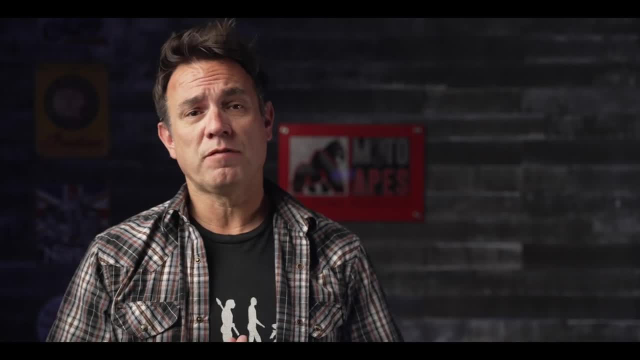 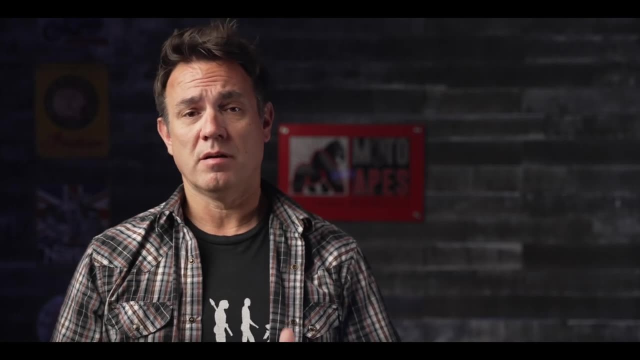 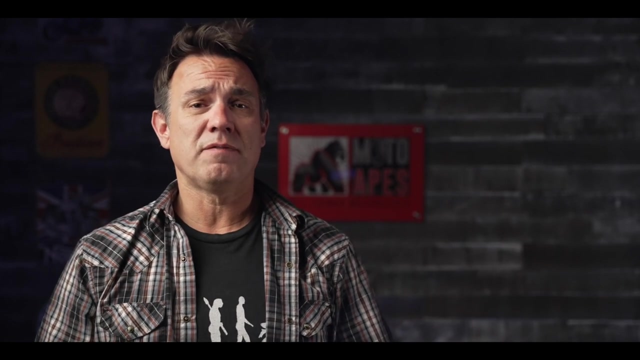 that occur at the scene of the crash. Thus, there is a need for more research on the nature, severity of injuries to riders, the characteristics of the associated crashes and the mortality rates both at the scene and in the hospital. We are then left with data and statistics that are available and as unscientific as it may be. 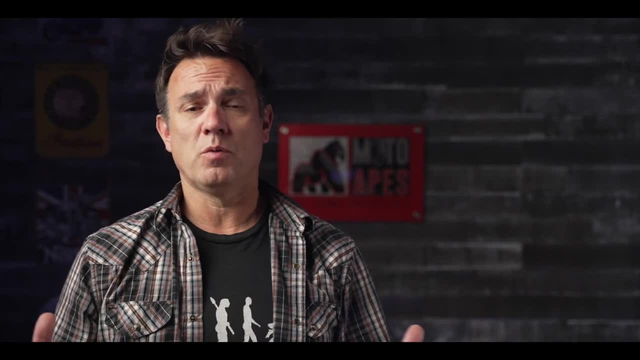 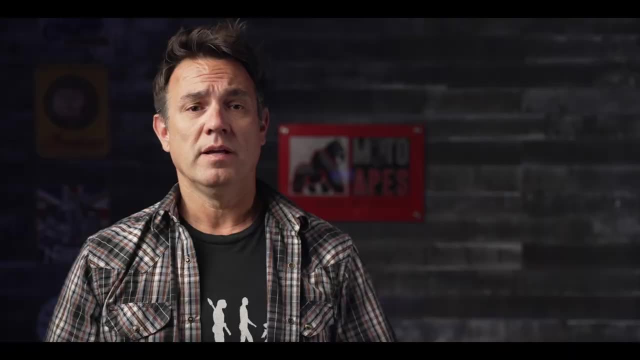 left to make our own conclusions. drawing an overall picture of motorcycle safety, Numerous statistical studies are available through PubMed that have been conducted over the past few decades as well. Data regarding rider demographics may have changed, but the injury types sustained by motorcyclists involved in injury types sustained by motorcyclists involved in. injury types sustained by motorcyclists involved in accidents has remained fairly static. So let's start here. The latest data from the NHTSA was released in September of 2021 and covers statistics for the year 2019.. Remember, this is the NHTSA report. 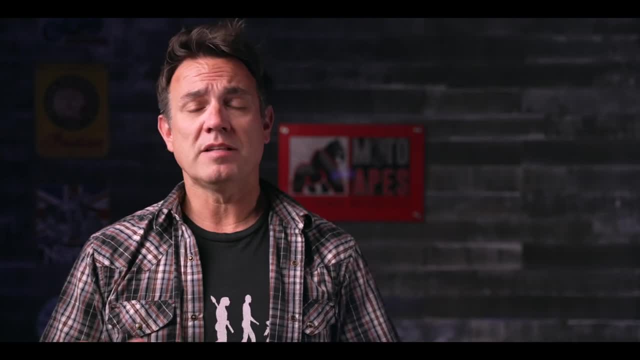 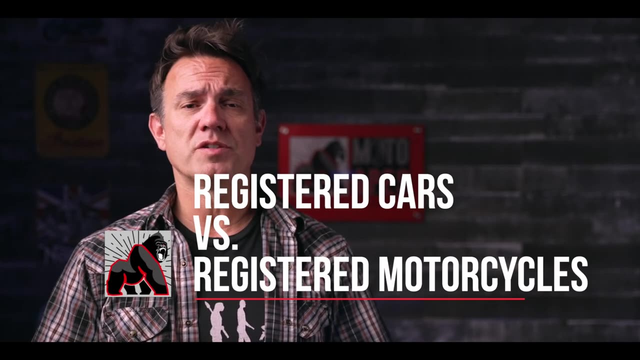 so these first stats are going to cover fatalities only, So let's start with stats and then deal with interpreting the data at the end. In 2020, the total number of public, personal and commercial motorcycles registered in the United States and the District of Columbia totaled approximately 8.32%. 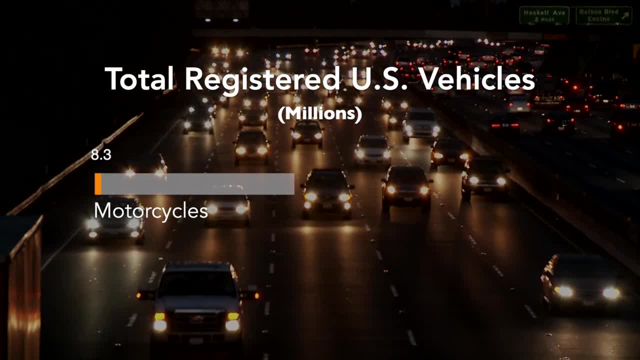 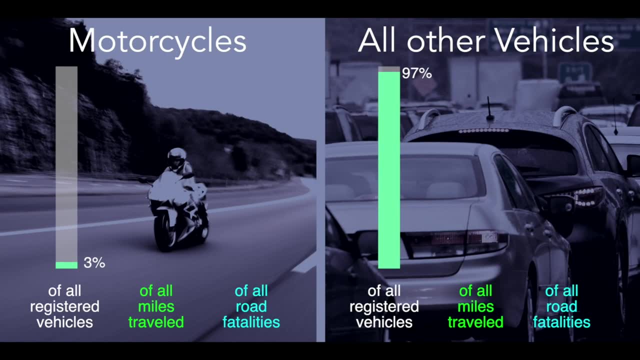 The number of registered vehicles which are not motorcycles in the United States is approximately 266.7 million. Although motorcycles make up only 3% of all registered vehicles and 0.6% of all vehicle miles traveled in the United States, motorcyclists accounted. 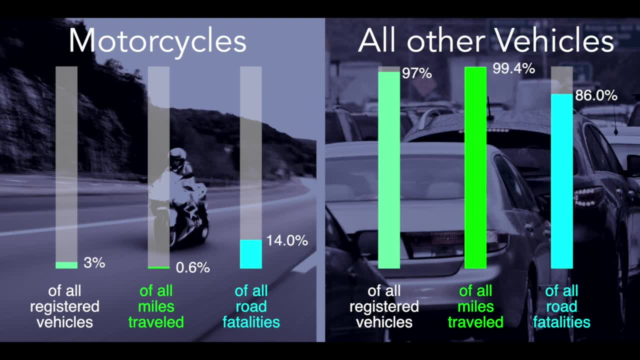 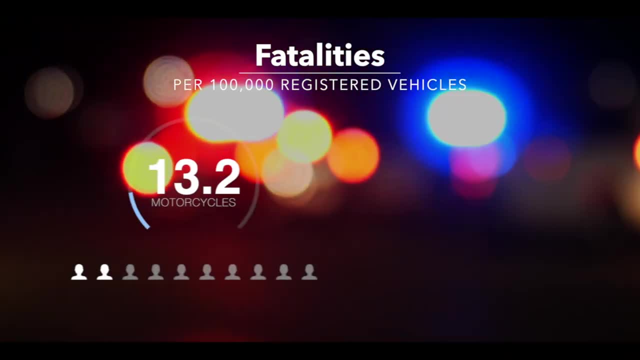 for 14% of all traffic fatalities, 18% of all occupant fatalities and 4% of all occupant injuries. The fatality rate per 100,000 motorcycles was 58.3 versus 9.4 for passenger cars. 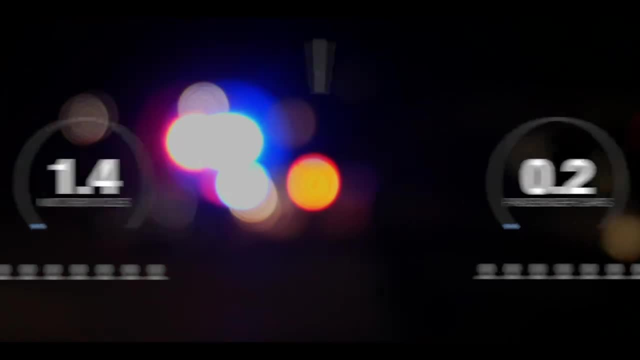 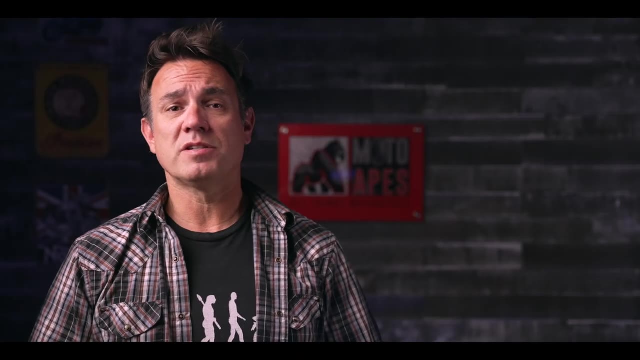 Per vehicle mile traveled. the fatality rate for motorcyclists was 29 times higher than that of passenger cars and 40 times higher than those of light trucks. The injury rate for motorcyclists was 4 times higher than that of passenger cars. 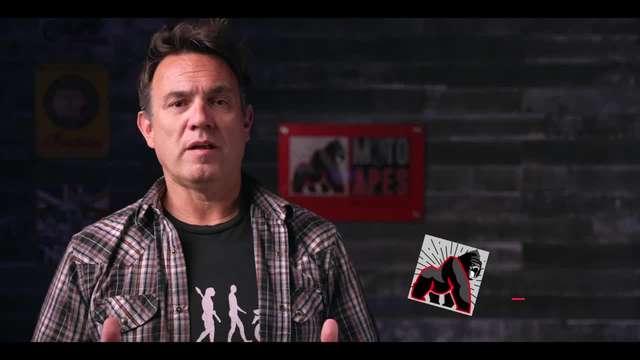 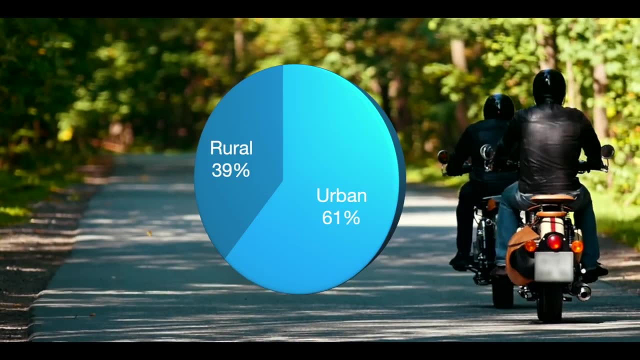 and 7 times higher than that of light trucks. So where are fatal motorcycle accidents occurring? 61% of the motorcycle fatalities occurred in urban areas, compared to 39% in rural areas. 66% occurred at locations that were not intersections, compared to 34%. 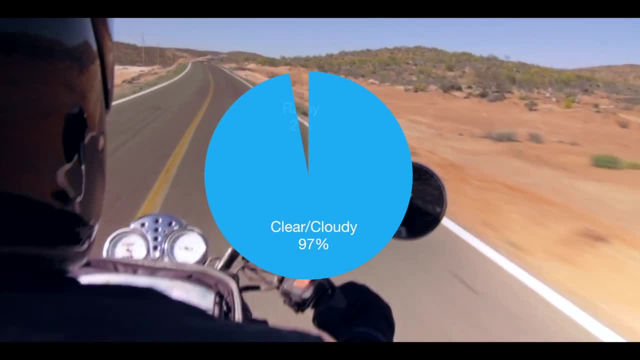 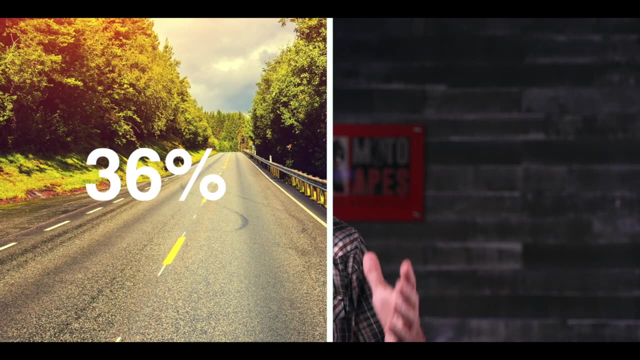 97% occurred in clear, cloudy conditions, compared to 2% in rain conditions and 1% in snow and sleet or fog. 57% occurred during the daylight, compared to 38% in the dark, 4% during dusk and 1%. during dawn, 91% occurred on non-interstate roads, compared to 9% on interstates. By Crash Type, The most harmful event in 2019, for 2,811 of the 5,114 motorcycles involved in fatal crashes, was collisions with motor vehicles in transit. 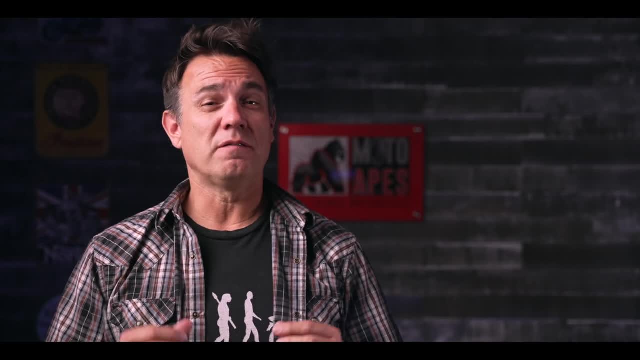 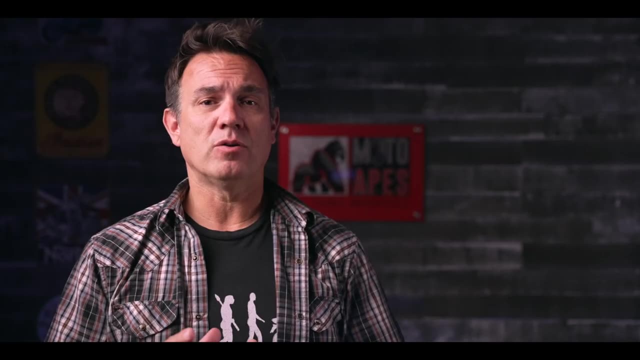 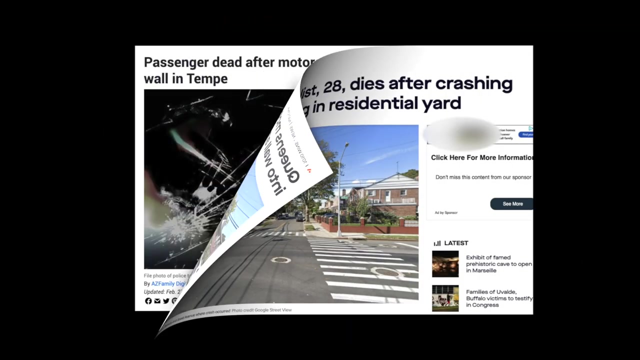 In two vehicle crashes. 76% of the motorcycles involved in fatal crashes were struck in the front. Only 7% were struck in the rear. Motorcycles were more frequently involved in fatal collisions with fixed objects than were any other vehicle type. 23% of motorcycles involved in fatal crashes in 2019 collided with fixed objects. 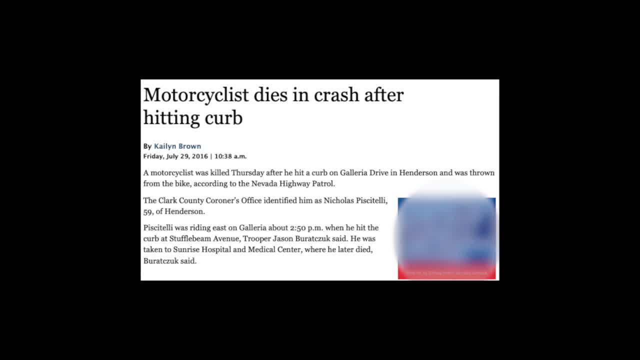 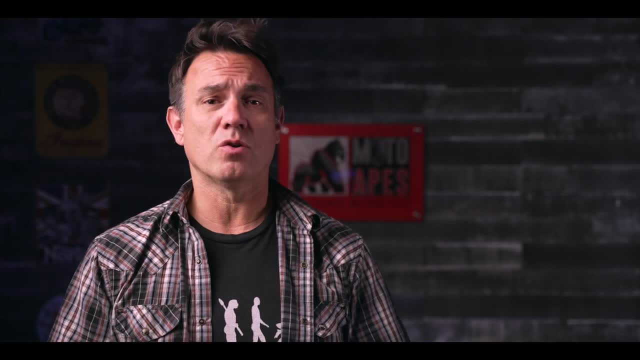 compared to 16% for passenger cars, 13% for light trucks and 4% for large trucks. In 2019, there were 2,495 fatal 2 vehicle crashes, each involving a motorcycle and another type of vehicle. 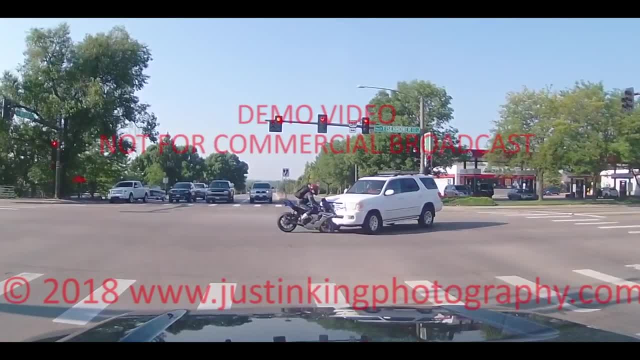 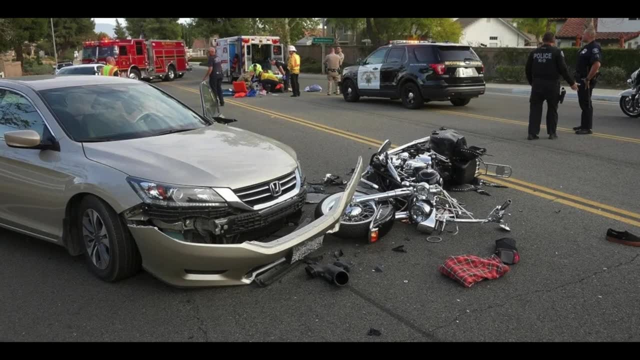 In 41% of these crashes, the other vehicles were turning left, while the motorcycles were going straight, passing or overtaking other vehicles. Both vehicles were going straight in 558 crashes. Here's an interesting one: 39.2% of all crashes were single. 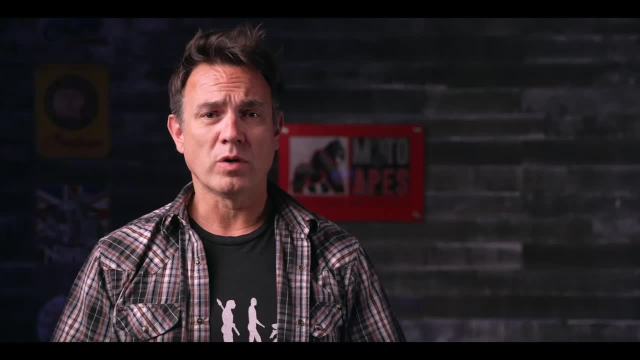 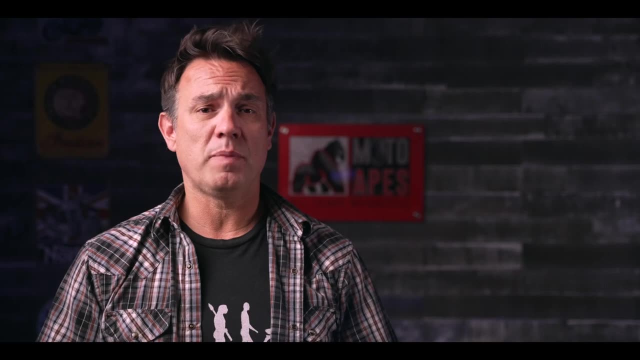 vehicle crashes where the motorcyclist lost control or poorly normalized them. Where the motorcyclist lost control or poorly negotiated a turn. In 1976, the NHTSA commissioned a study that led to the publishing of the 452-page Hurt Report, Named after its primary author, University of Southern California professor. 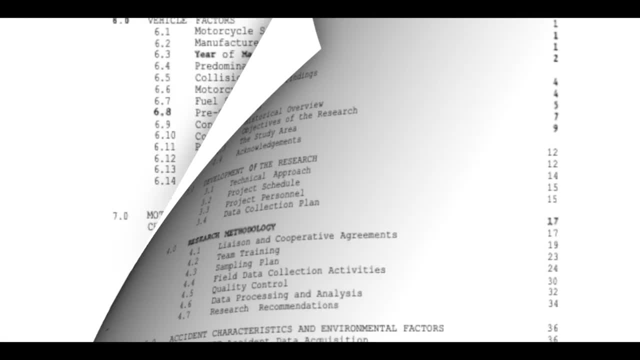 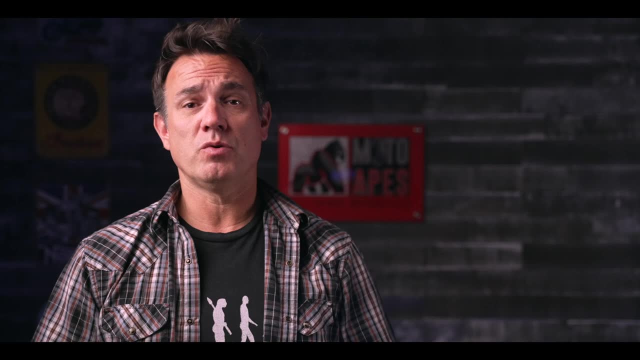 Harry Hurt. the 435-page study is still considered to be the benchmark study into motorcycle safety and accident prevention, Though some insights and observations made in the Hurt Report remain true some 40 years later. one interesting change that has occurred is in the age group of riders killed. in motorcycle accidents During the five years observed for the Hurt Report, riders 16 to 24 had significantly more accidents, factored by the sampled age demographic, than all other age groups During that same period. riders 30 to 50 had much, much less. But fast forward to 2019,. 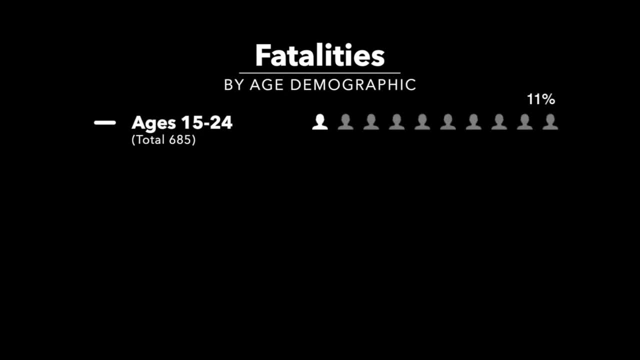 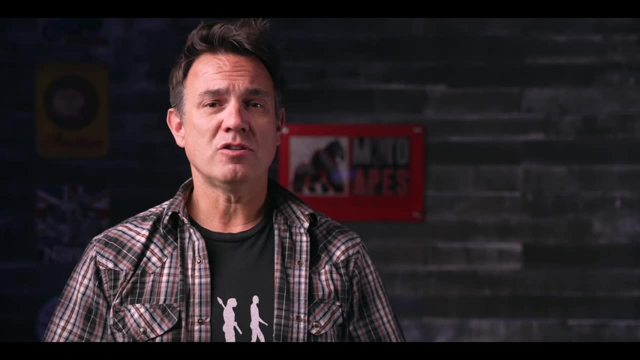 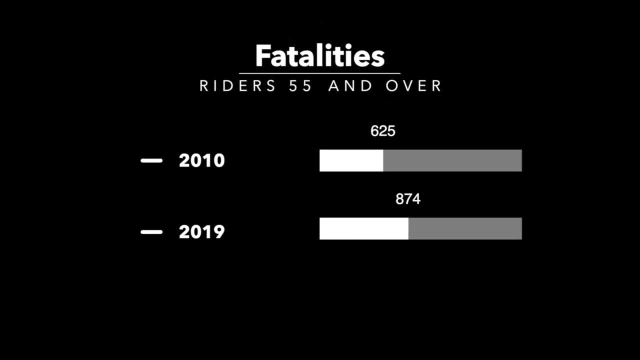 and for the age group 15 to 24, there were 685 fatalities, and age group 30 to 50 had a total of 1,763 fatalities. Most interestingly from the NHTSA report is the 55 and older age groups rise in fatalities Over the 10-year period from 2010 to 2019,. 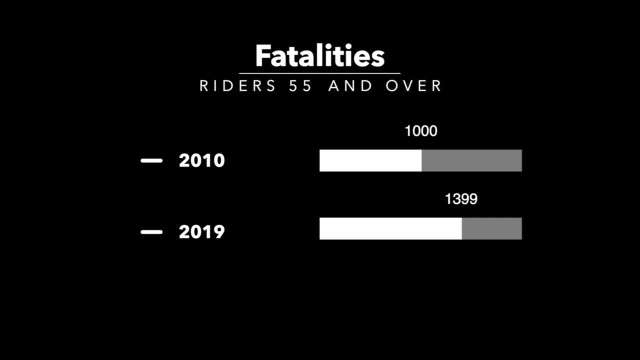 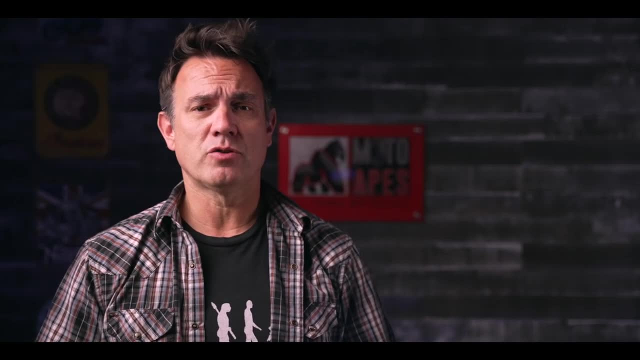 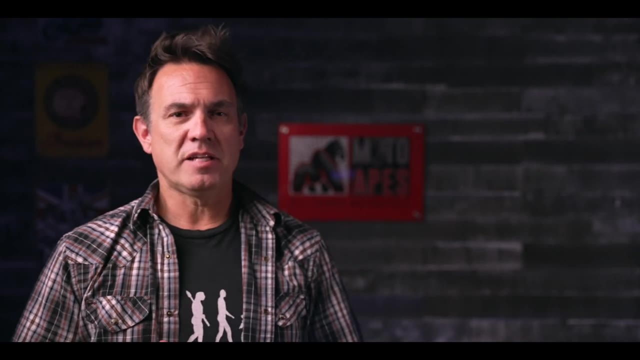 motorcyclist fatalities amongst the 55 and older age group increased by 40 percent from 1,000 to 1,399.. In 2010,, the average age of motorcycle riders killed in traffic crashes was 42, whereas in 2019, the average age bumped up to 43.. The NHTSA published fatality data for age. 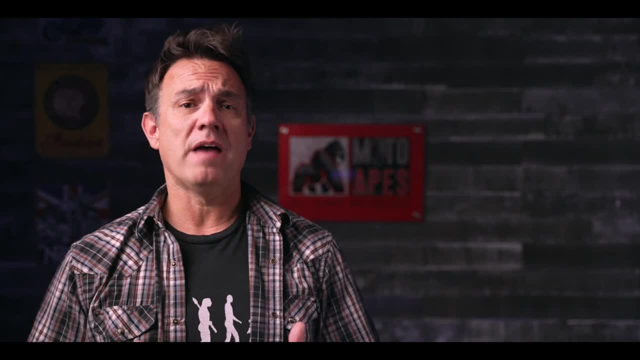 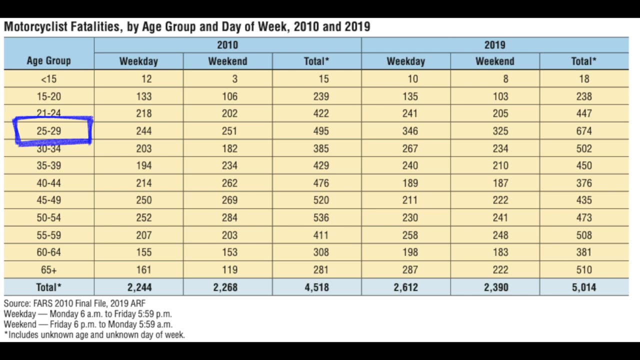 groups 15 and under, and then divided the remainder of age groups in five-year increments until reaching ages 65 and above. The 25 to 29-year-old motorcyclist age group had the highest number of fatalities, at 674,, 13 percent of all fatalities for the year. 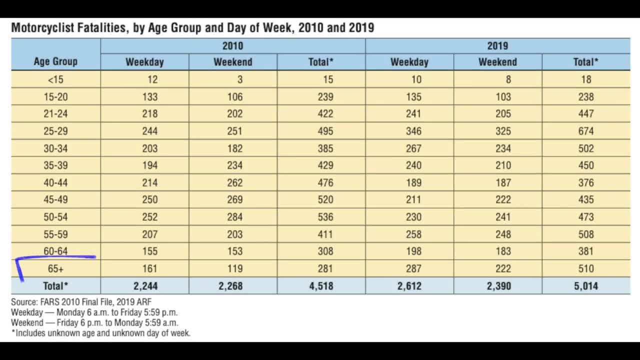 It surprised me to learn that the 65 and older age group accounted for the next highest fatality number of 510 riders. This was followed closely by 55 to 59 at 508.. During 2019, roughly half the accidents that killed motorcyclists occurred during the weekend, versus the weekday. 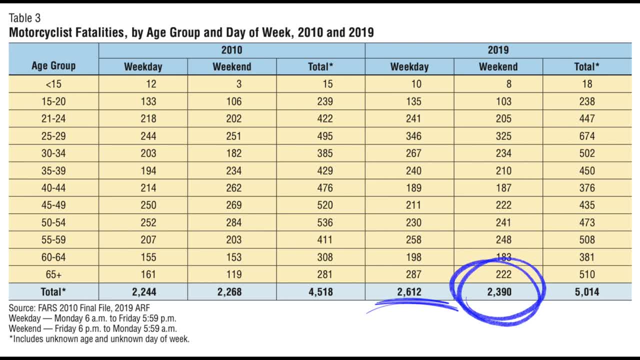 Additionally, the NHTSA published fatalities for the age group 55 to 59, and the average age group fatalities on weekdays increased by 16 percent from 2,244 in 2010 to 2,612 in 2019.. 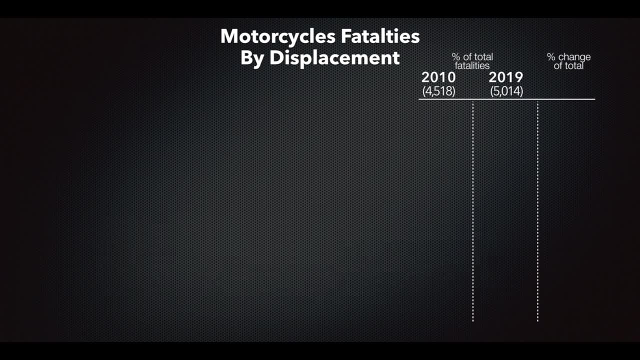 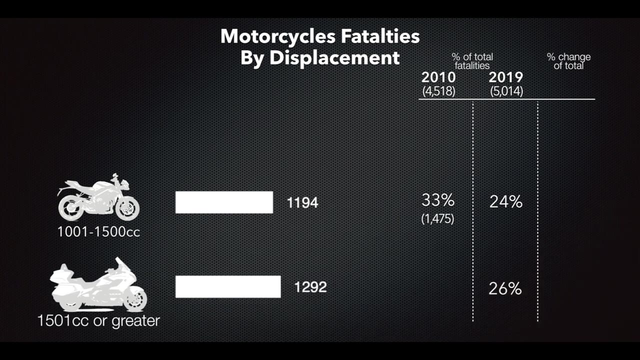 24 percent of motorcyclists killed in traffic crashes in 2019 were riding motorcycles with engine sizes from 1,001 to 1,500 cubic centimeters, down from 33 percent in 2010.. 26 percent of motorcyclists killed in 2019 were riding motorcycles with engine sizes of 1,501 cc or up. 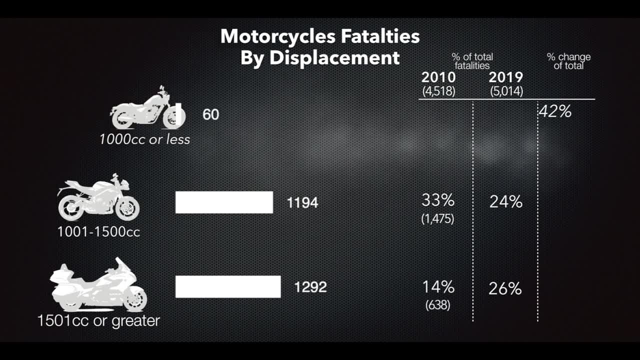 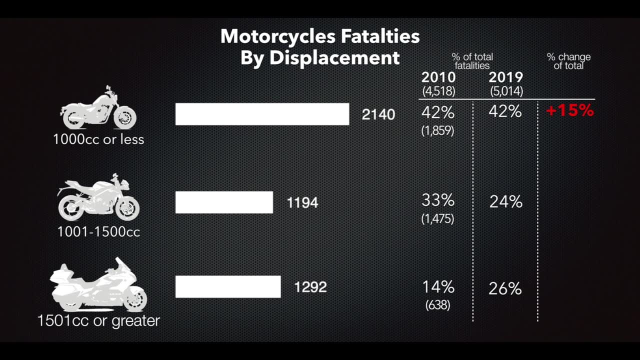 up from 14 percent in 2010.. The number of motorcyclist fatalities on motorcycles with engine sizes of 1,000 cc or less showed an increase of 15 percent. during this time, Motorcyclist fatalities on motorcycles with engine sizes between 1,001 and 1,500 cc actually decreased by 19 percent, while the 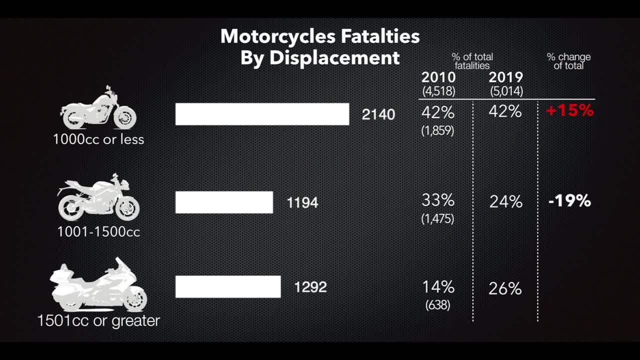 number of motorcyclists killed on motorcycles with engine sizes 1,501 cc or higher increased by 103 percent from 638 to 1,292 riders. We can't talk accident statistics, but we can talk about statistics without talking speed when it comes to motorcycles. 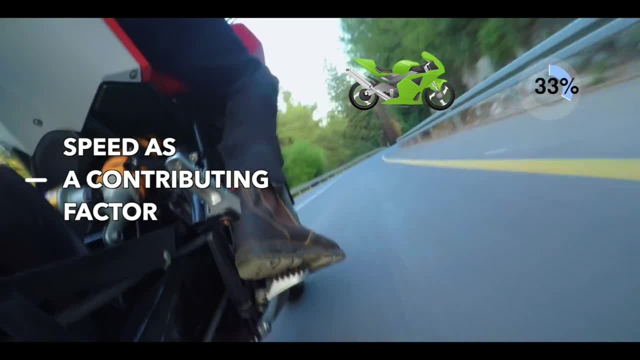 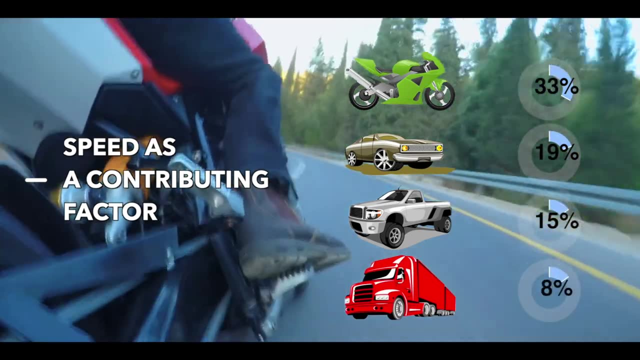 33 percent of all motorcycle riders involved in fatal crashes in 2019 were speeding, compared to 19 percent for passenger car drivers, 15 percent for light truck drivers and 8 percent for large truck drivers. Motorcycle riders 21 to 24 years old involved in fatal crashes. 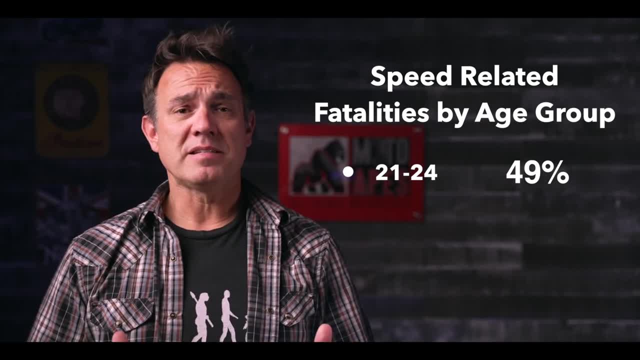 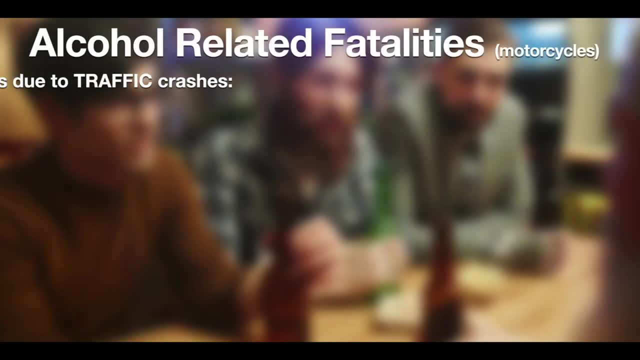 had the highest speeding involvement, at 49 percent. Not surprisingly, riders aged 64 and up had the lowest fatality rate due to speeding. Alcohol In 2019, there were 4,000 people who died in a car crash in 2019.. In 2019, there were: 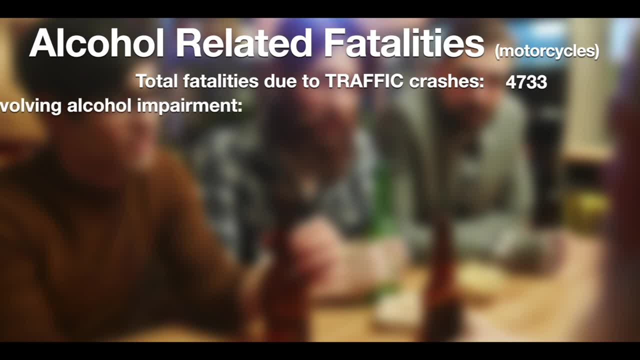 1,733 motorcycle riders killed in traffic crashes. Of those, 1,383 were alcohol impaired with a blood alcohol content of .08 or higher. In addition, there were 354 motorcycle riders killed who had lower alcohol levels, or BACs, of .01 to .07.. 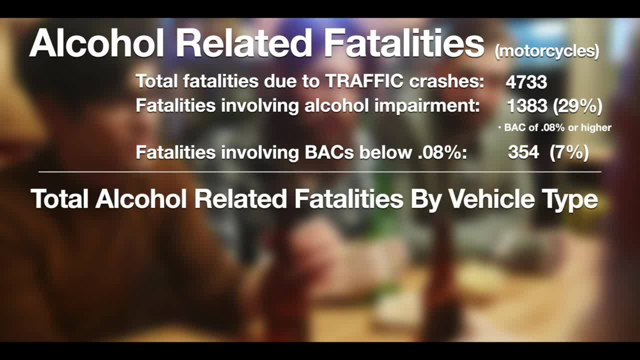 Motorcycle riders involved either killed or survived in 2019 had higher percentages of alcohol impairment than any other type of motor vehicle driver: 29 percent for motorcycle riders, 1 percent for passenger cars, 19 percent for light trucks and 2 percent for large trucks. 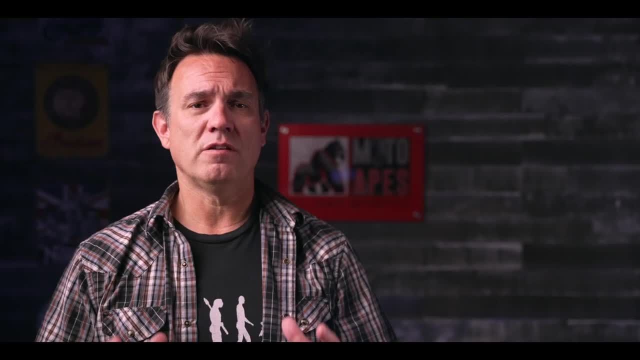 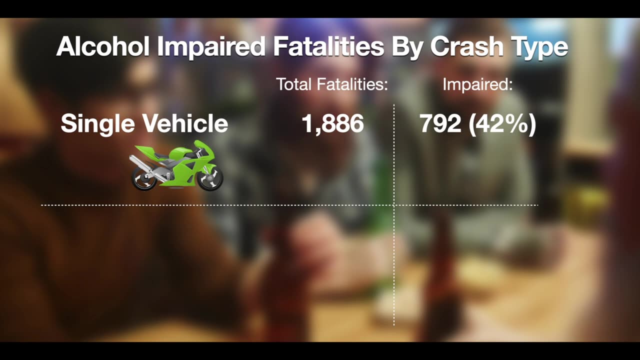 The highest percentages of alcohol impaired motorcycle rider fatalities were in the 40 to 44 age group. 42 percent of the 1,886 motorcycle riders who died in single vehicle crashes in 2019 were alcohol impaired, as compared to 21 percent of the 2,847 motorcycle riders who died in. 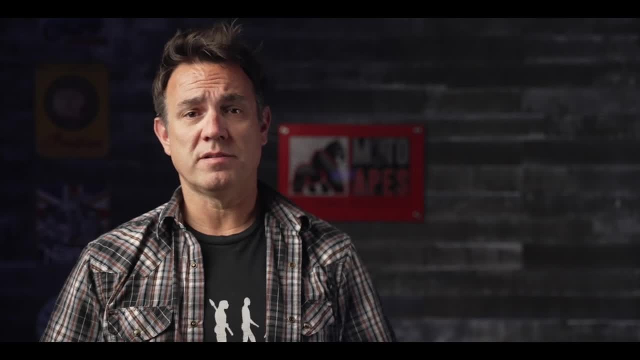 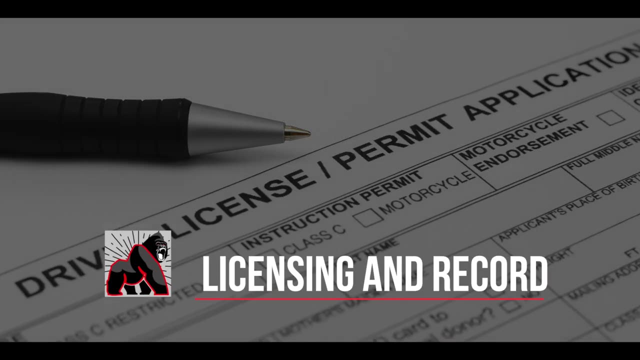 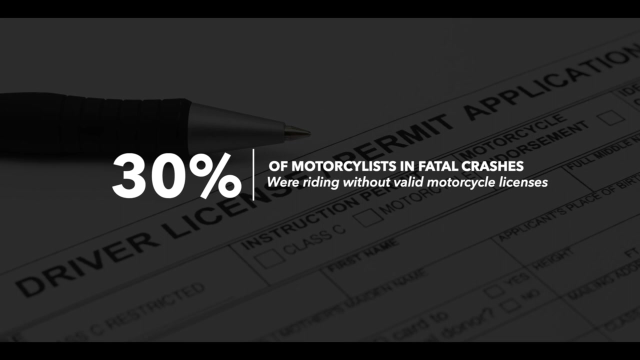 multiple vehicle crashes. 48 percent of those killed in single vehicle crashes on weekends in 2019 were alcohol impaired Licensing and Prior Driver Records. 30 percent of motorcycle riders involved in fatal crashes in 2019 were riding without valid motorcycle licenses at the time of the crashes, while only 13 percent of passenger 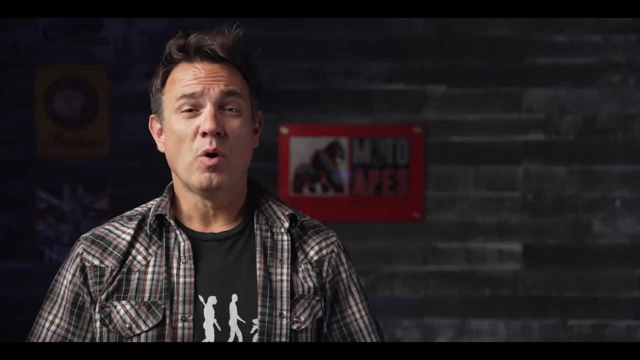 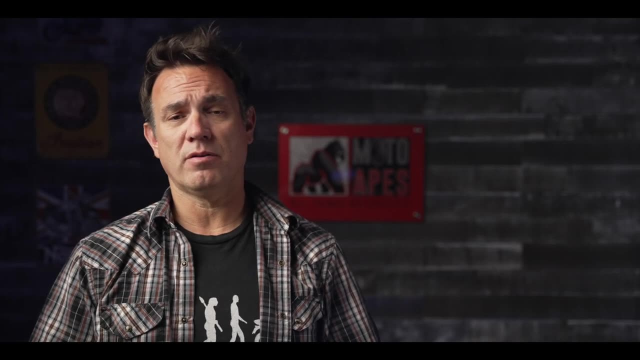 vehicle drivers in fatal crashes did not have valid licenses. Motorcycle riders involved in fatal crashes had the highest percentage of drivers with previous driving records as compared to any other vehicle driver. Motorcycle riders involved in fatal crashes were 1.4 percent of those killed in single vehicle crashes on weekends. The highest percentage of motorcycle riders involved in fatal crashes had the highest percentage of vehicles in fatal crashes. tend to be 4 or 8 percent of the older of their ubiquity enriching motor deaths of any model. over 200,000 people were on long distance vehicle. 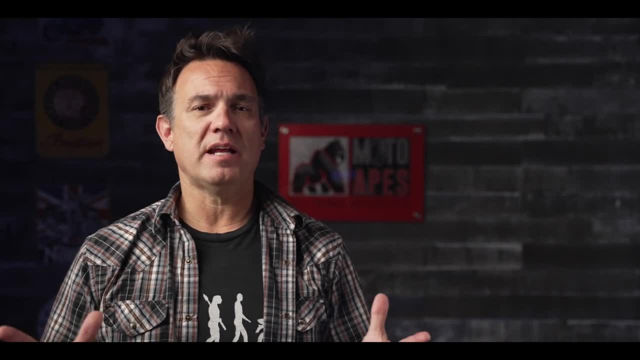 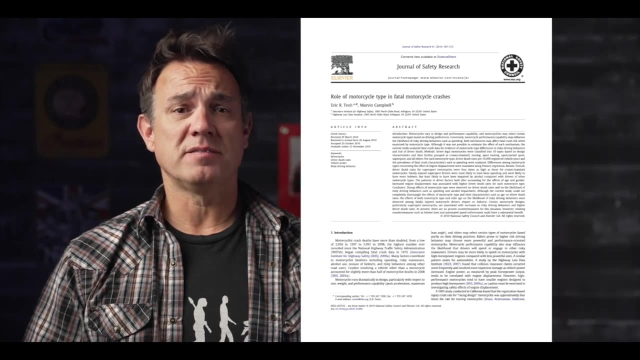 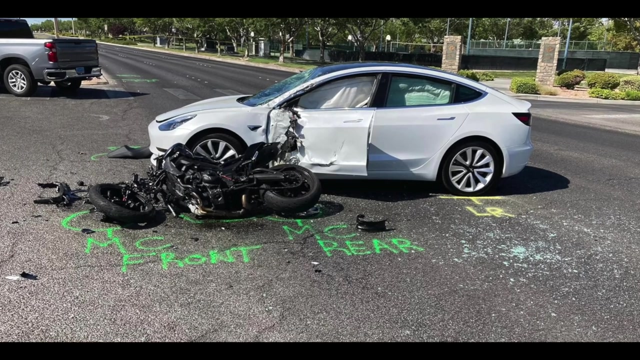 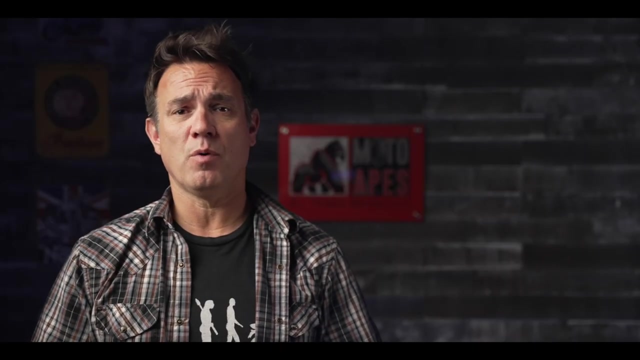 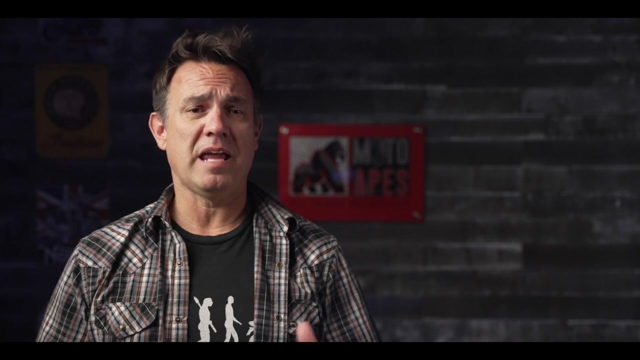 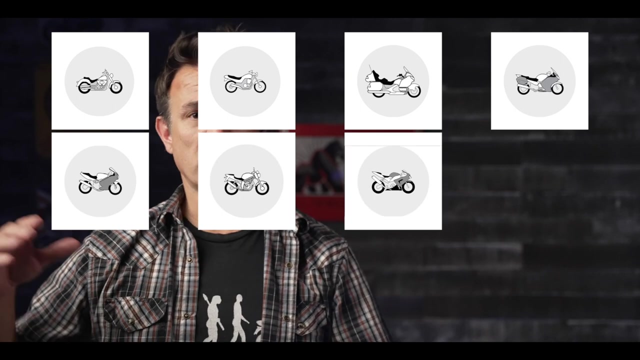 crashes. imental related bikes. Motorcycles were grouped into 12 types based on a classification system developed by the HLDI Cruiser Standard: Touring Sport- Touring Sport Unclad Sport- Super Sport, Chopper. 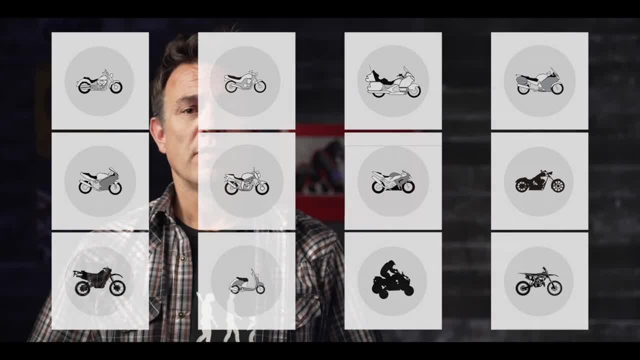 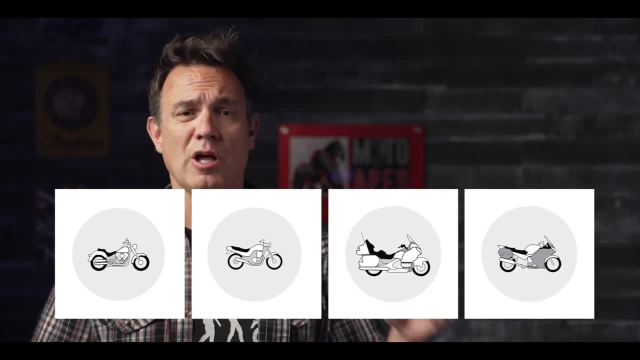 Dual Purpose Scooter and All-Terrain Vehicle or Off-Road. The report found that these death rates indicate the drivers of Cruisers. Standards Touring and Sport Touring motorcycles have the lowest death rates. Super Sport motorcycles make up a small fraction of registered motorcycles. 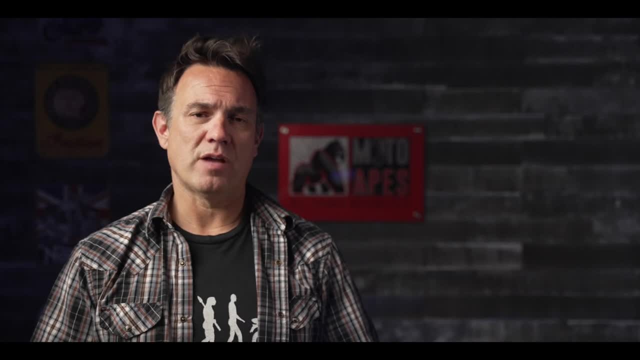 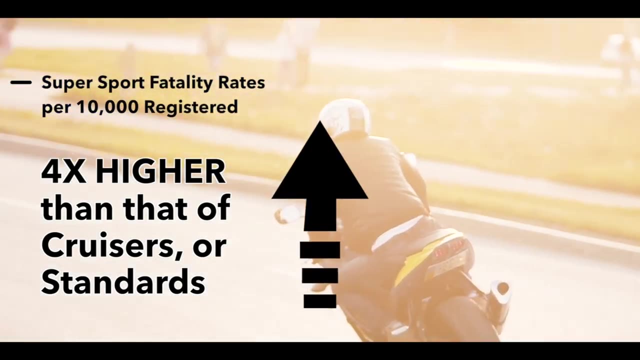 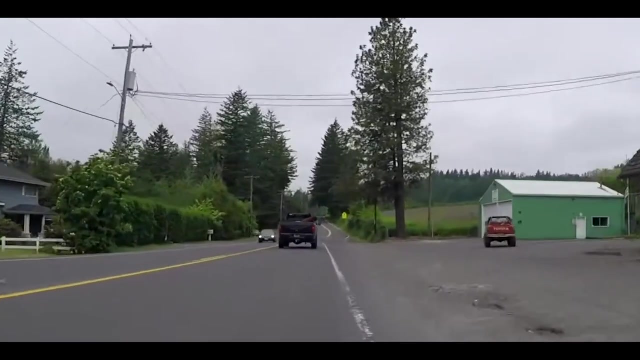 but their riders are overrepresented in fatal crashes. The study found that the driver death rate per 10,000 registered motorcycles for Super Sports was about four times as high as the rate for motorcyclists who rode Cruisers or Standards. Motorcycle performance capability may influence. 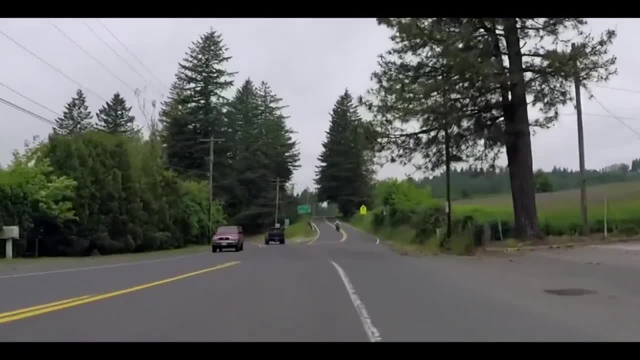 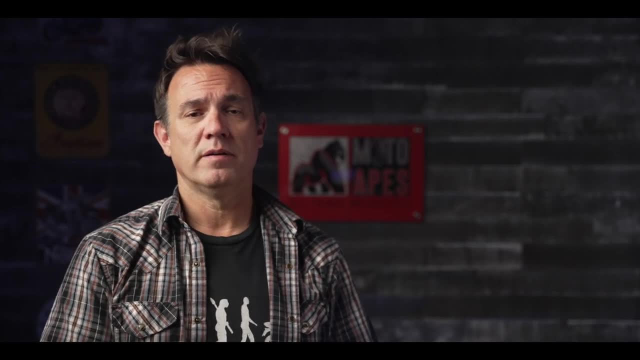 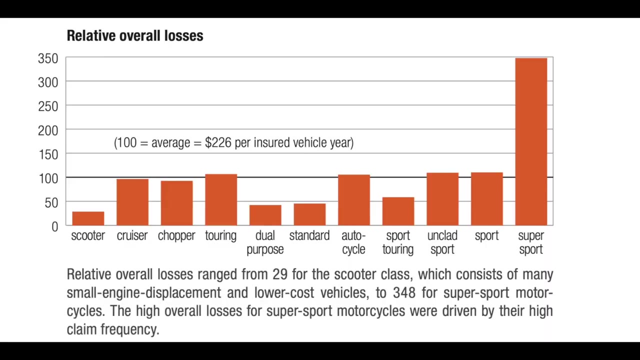 the likelihood that drivers will speed or engage in other risky maneuvers. Drivers may be more likely to speed on motorcycles with high horsepower engines compared with less powerful ones. Now, a similar pattern exists. A study by the Highway Loss Data Institute, or the HLDI I mentioned earlier, found that collision 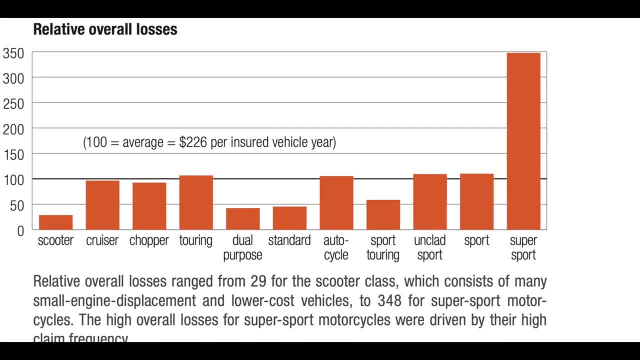 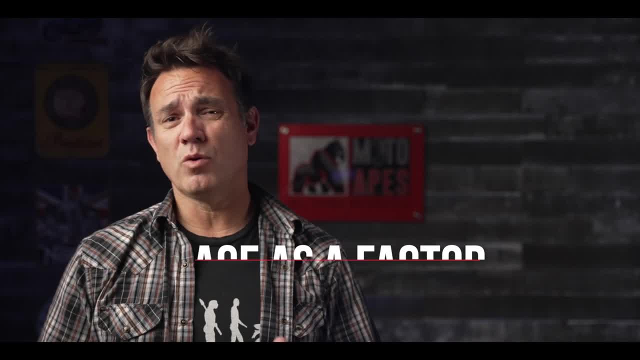 insurance claims occurred more frequently and involved more expensive damage as vehicle power increased. Injuries in riders' ages: Although the NHTSA report gives an estimate of motorcyclists injured in 2019 of about 84,000, there is no data on the types of injuries. motorcyclists are more. 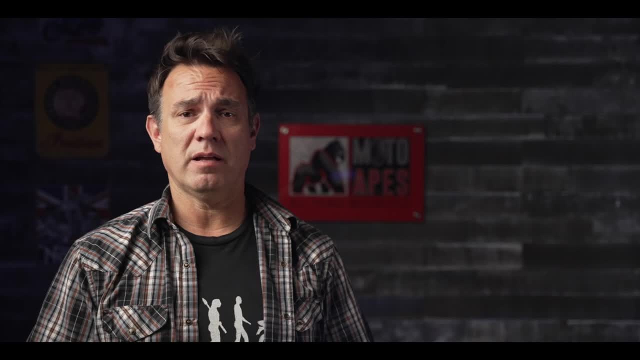 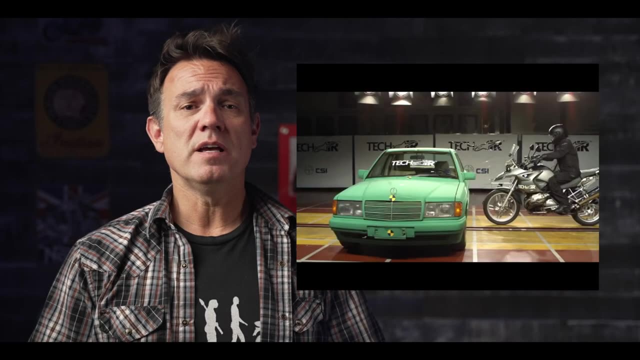 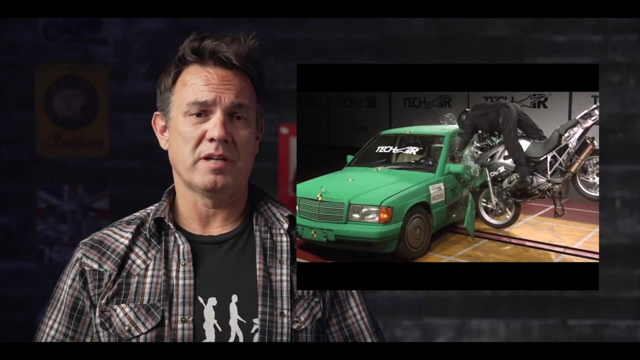 likely to incur and to what extent those injuries would lead to fatality. The HURT report remains one of the best studies to reference injury status. Even though safety gear has certainly improved since the publishing of the report, injury type has probably not changed that significantly due to the nature of a motorcycle accident. The first and probably somewhat obvious statistic of the 900 accidents surveyed in the HURT report is that 98% of all motorcycle accidents result in some form of injury to the rider. To be fair, the high rate of injury observed in the report may be high since accident. 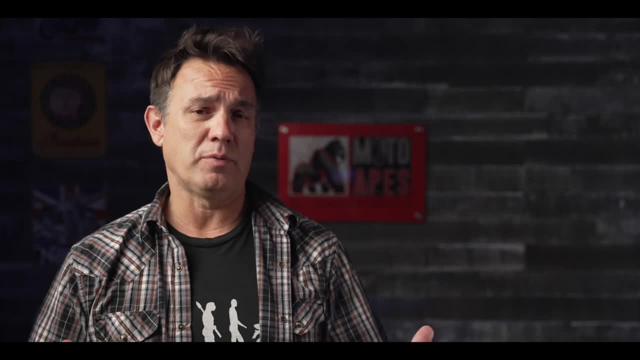 notification was dependent primarily upon dispatch of a rescue ambulance. The HURT report has shown that motorcyclists are more likely to incur and to what extent the accident could lead to fatality. The HURT report lists extremities as the most common form of severe 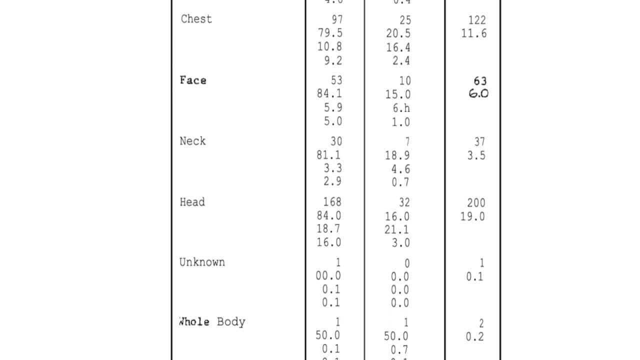 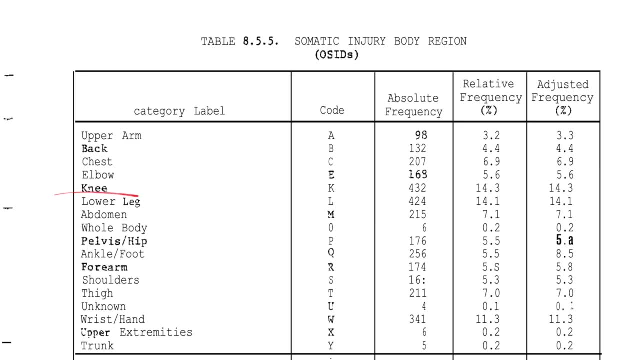 injury to riders at 45%, followed by head at 19% and chest at 12%. Getting more specific, the HURT report documents: the most common injuries to the extremities were the knee at 14.3%, the lower leg at 14.1%, followed by the wrist and hand at 11.9%. A report published in 2006. 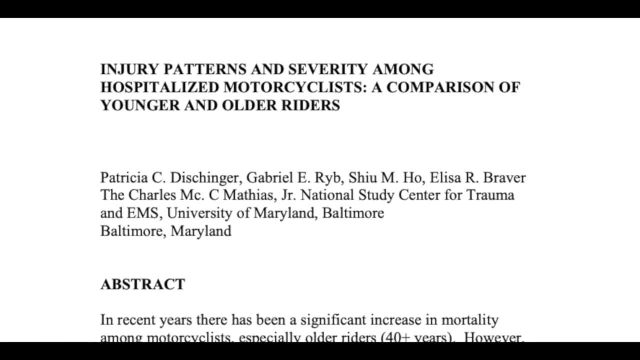 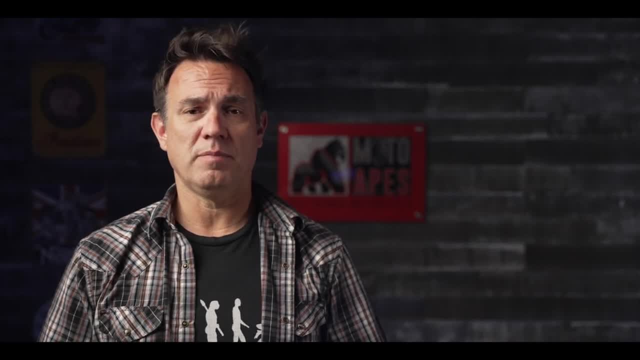 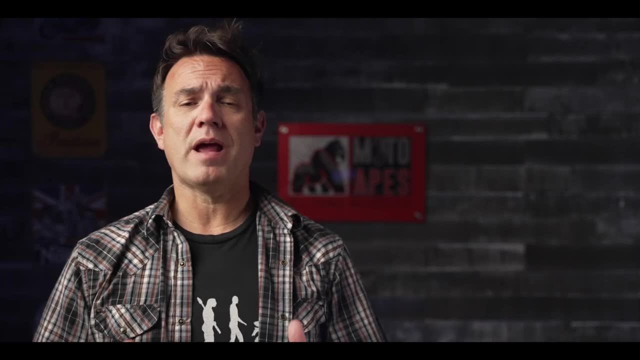 titled Injury Patterns and Severity Among Hospitalized Motorcyclists- a comparison of younger and older riders adds a little more light on the types of injuries that are more likely to be fatal and the incidence difference between younger and older riders, Although the study only accounts for riders hospitalized and not riders who died at the scene. 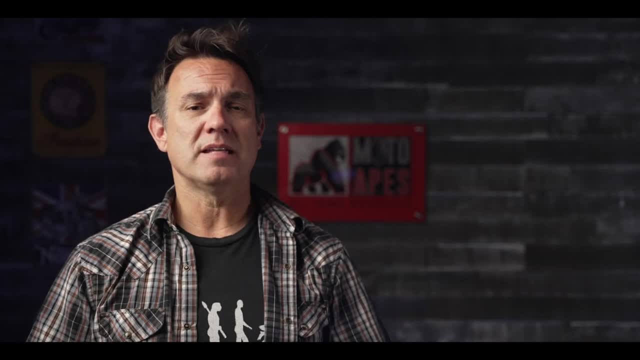 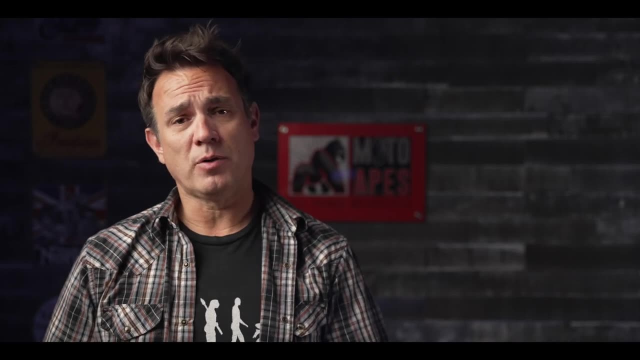 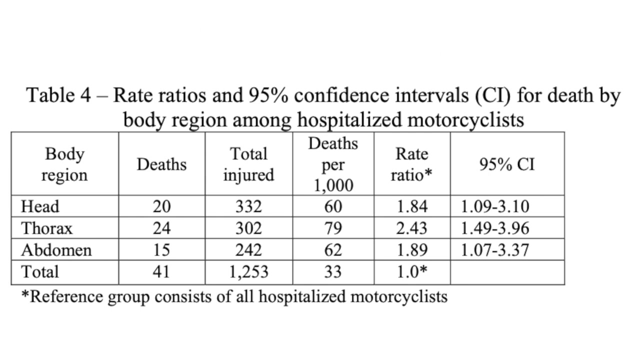 it paints a pretty clear picture. Among those hospitalized, significant increases in mortality were observed among motorcyclists who had head injuries, thoracic injuries and abdominal injuries, with the highest risk occurring. amongst the group with thoracic injuries, The order of morbidity was thorax, head and abdomen. The study generated some other interesting 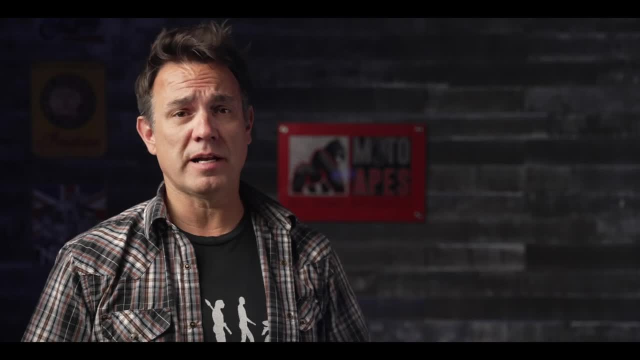 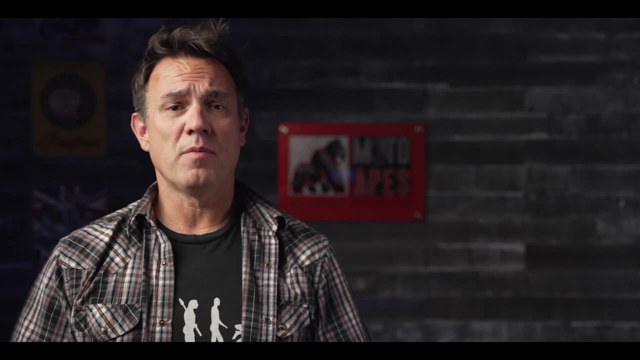 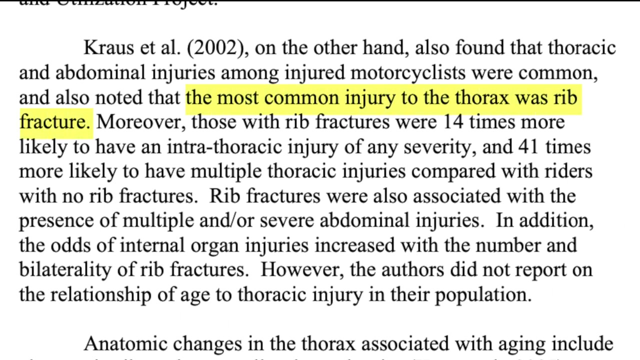 observables. It characterized riders into groups younger and older. It cites a few other published reports stating thoracic and abdominal injuries among injured motorcyclists were common and also noted that the most common injury to the thorax was rib fracture- Those with rib 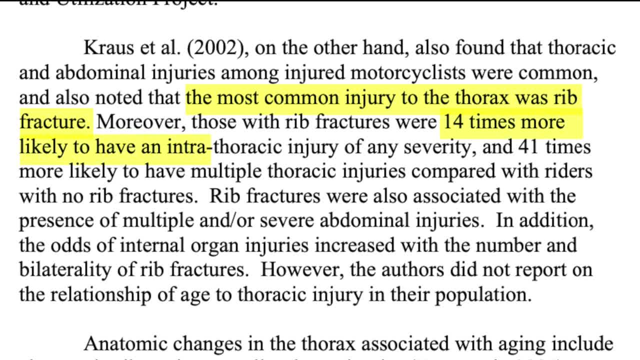 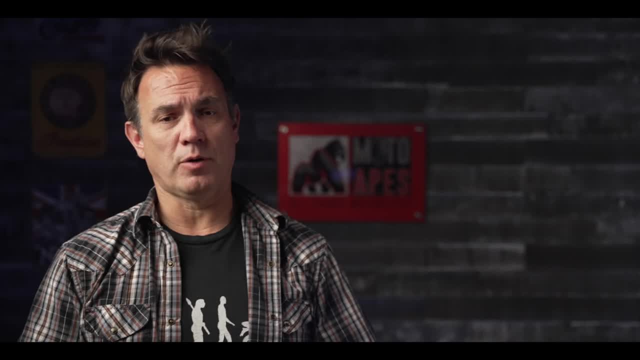 fractures were 14 times more likely to have an intrathoracic injury of any severity and 41 times more likely to have multiple thoracic injuries, compared with riders with no rib fractures. Rib fractures were also associated with the presence of multiple and or severe abdominal 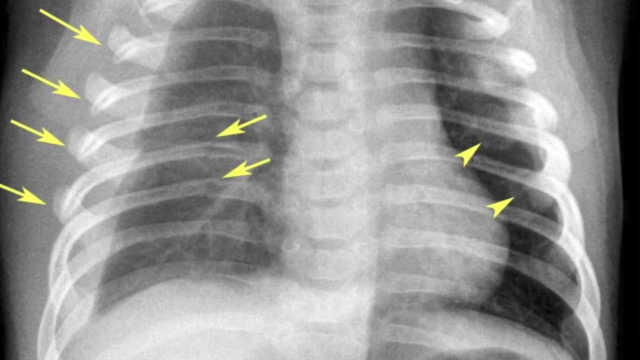 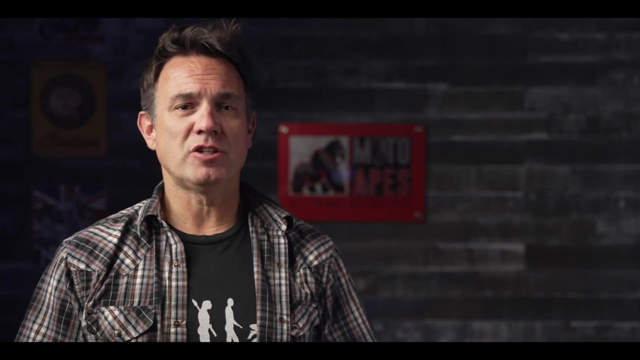 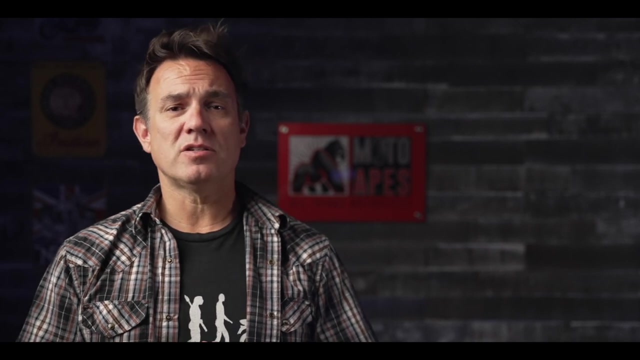 injury. In addition, the odds of internal organ injury increased with the number and bilaterality of rib fractures. With specific reference to age, the report states anatomic changes in the thorax associated with aging include changes in rib angles as well as bone density. Perhaps these changes contribute to the greater 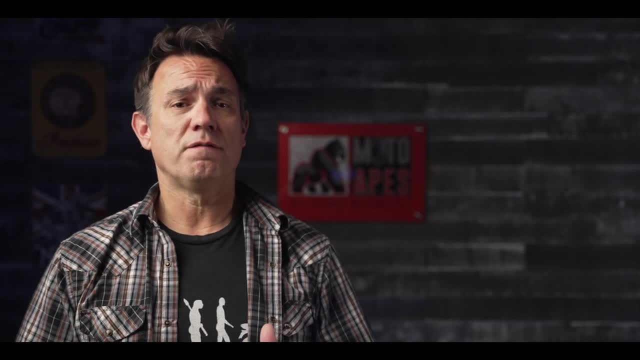 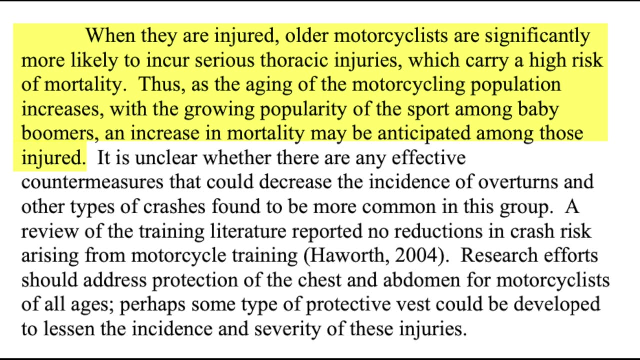 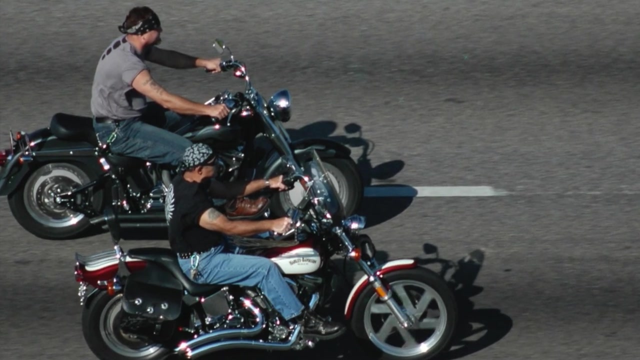 risk of rib fractures in the older group. There are also physiological changes in pulmonary compliance which also may place older motorcyclists at higher risk of complications following serious thoracic injury. Helmets: The debate between Kentucky and the rest of the world rages on The NHTSA estimates. 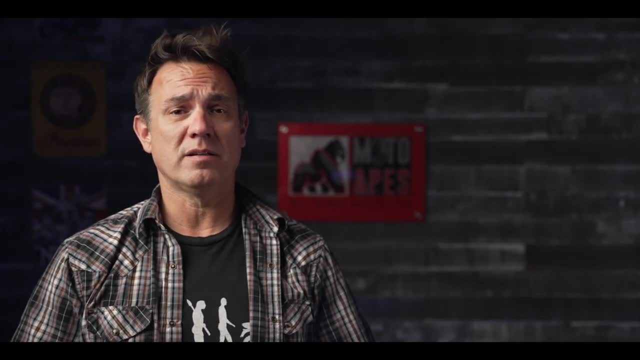 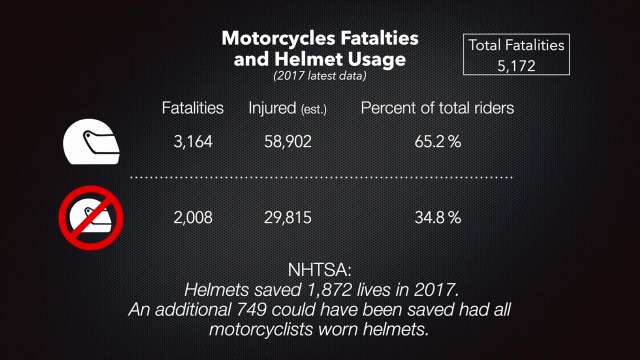 that helmets saved the lives of 1,872 motorcyclists in 2017.. If all motorcyclists had worn their helmets, an additional 749 lives could have been saved. Helmets are estimated to be 37 percent effective in preventing fatalities to motorcycle riders and 41 percent 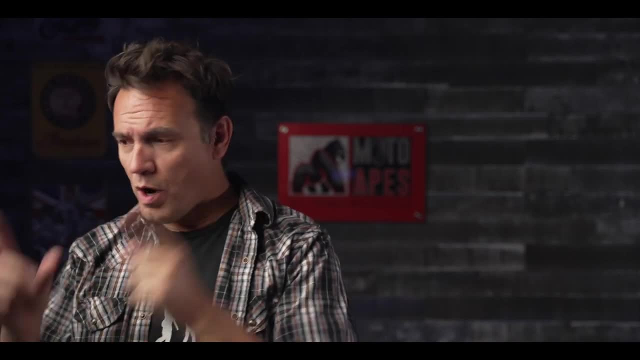 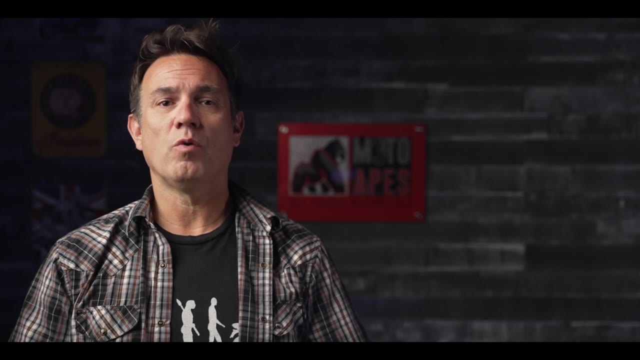 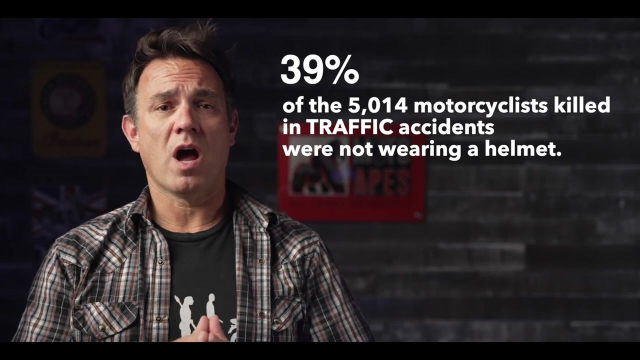 for motorcycle passengers. In other words, for every 100 motorcycle riders killed in crashes while not wearing helmets, 37 of them could have been saved had all 100 worn their helmet. 39 percent of the 5,014 motorcyclists killed nationwide in traffic crashes were not 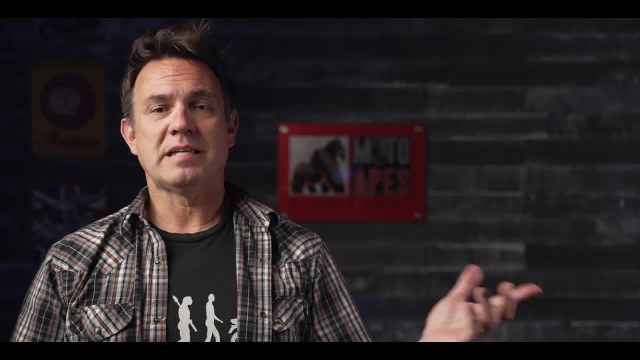 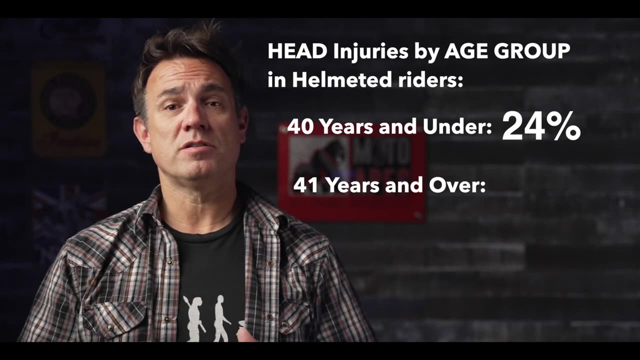 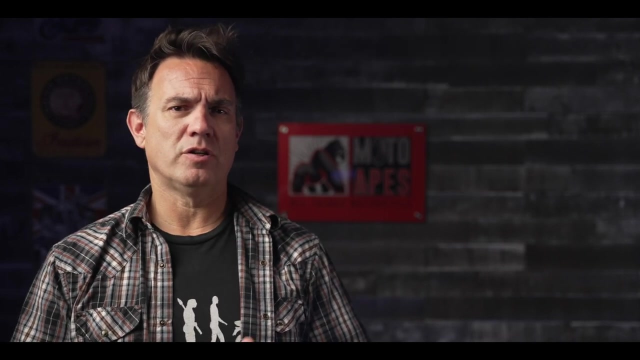 helmeted. For those of you that love data, back to the Tal and Campbell report. 24 percent of riders under the age of 40 who were helmeted experienced head injuries, versus 31 percent of helmeted riders over the age of 40. Younger riders with helmets had fewer head and facial injuries. 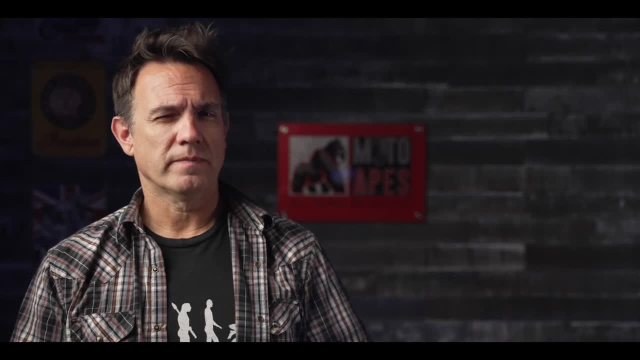 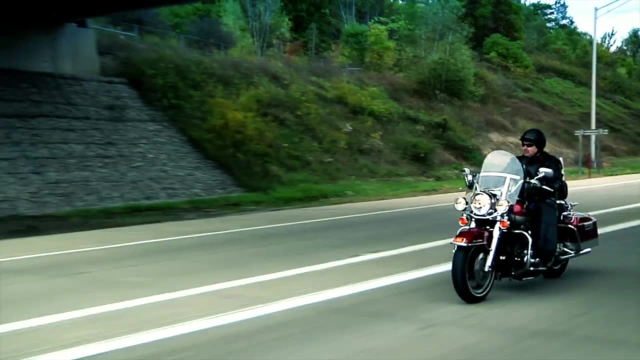 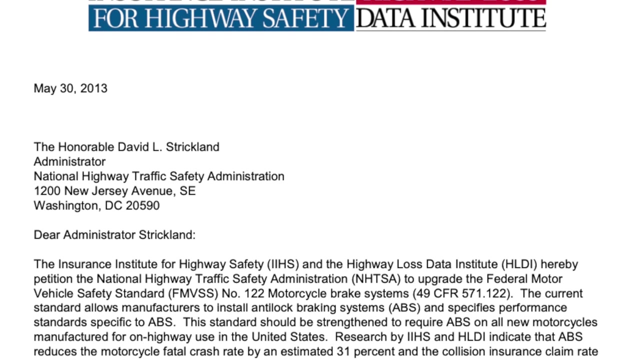 whereas older riders with helmets had more such injuries. It's unknown whether there were differences in types of helmets worn by the two age groups based upon the data collected, but I think we can make our own conclusions here. Let's talk about ABS, Nearly a decade after the Insurance Institute for Highway Safety. 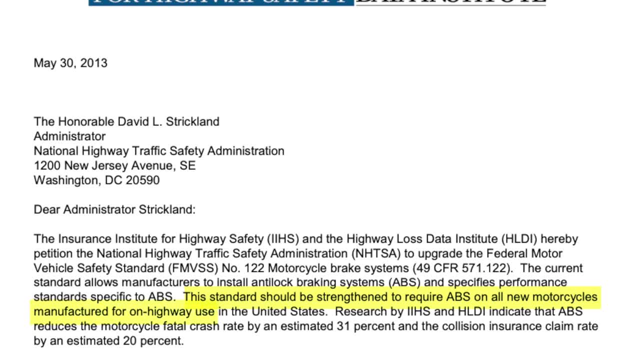 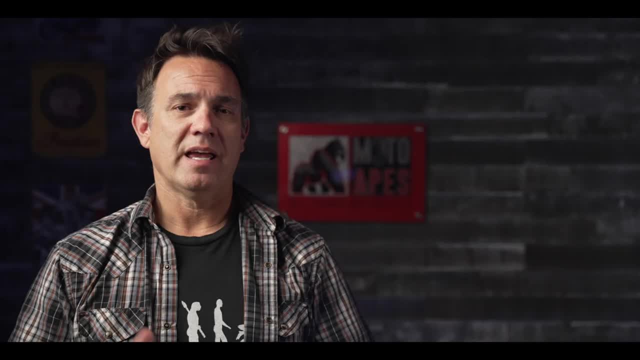 first called for a federal mandate requiring street-legal motorcycles to be equipped with anti-lock braking systems. the data continues to pile up in favor of this life-saving technology, Examining fatal crash rates for 65 motorcycle models offering ABS as an option over 2013 to 2019,. 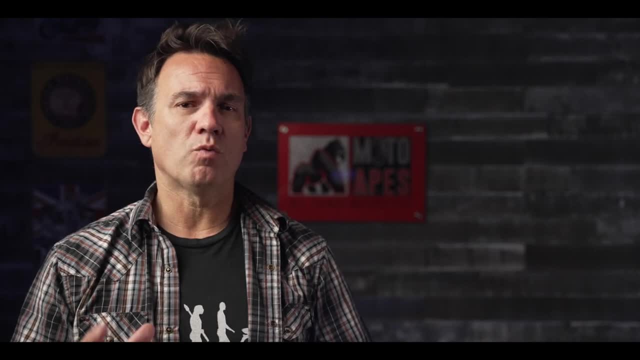 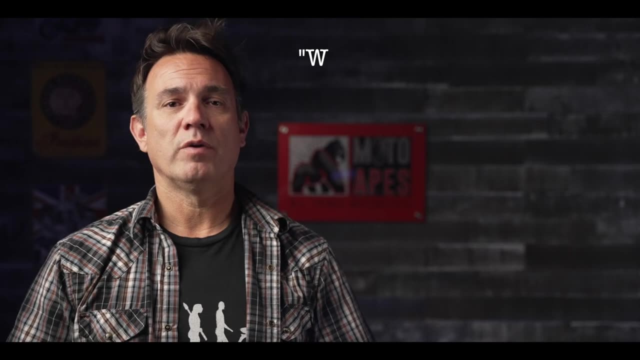 the researchers found that bikes equipped with the feature were involved in 22 percent fewer fatal crashes per 10,000 registered vehicles. The report states, quote: when it comes to decisions riders can make to protect themselves, choosing ABS is right up there with wearing a helmet. 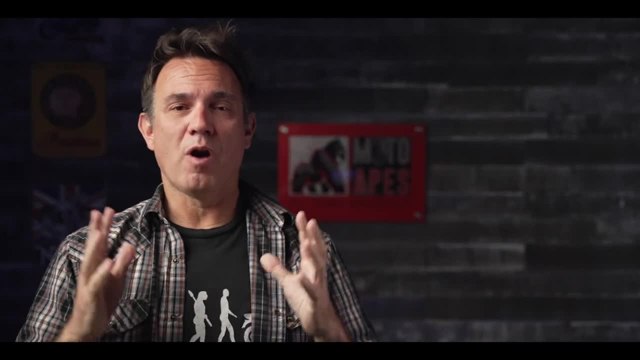 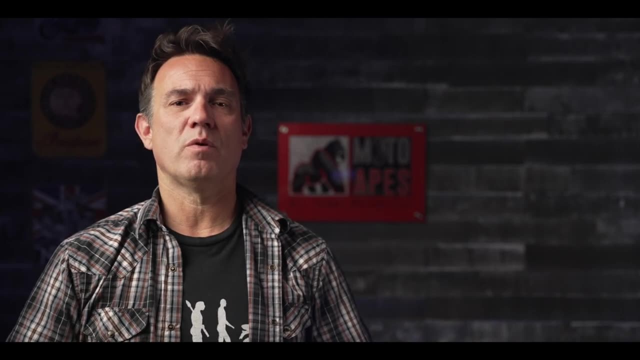 By now we're up to our ears in statistics and facts, and while motorcycle technology has changed and added some new safety features like ABS, it's pretty clear we are all taking a certain risk when we throw our legs over any motorcycle. Risk mitigation then becomes paramount when 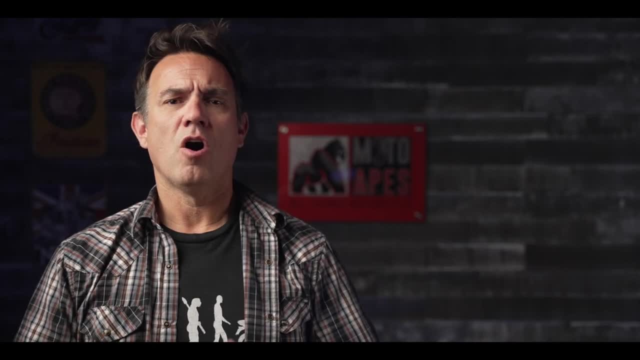 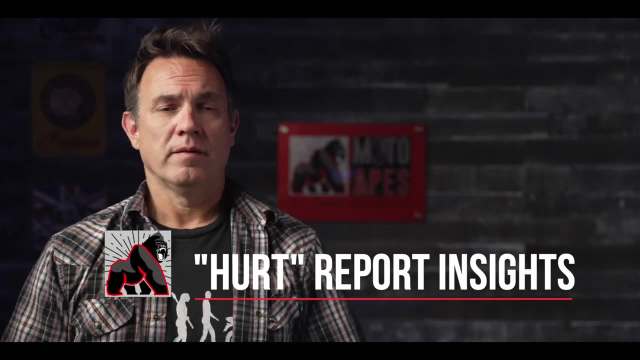 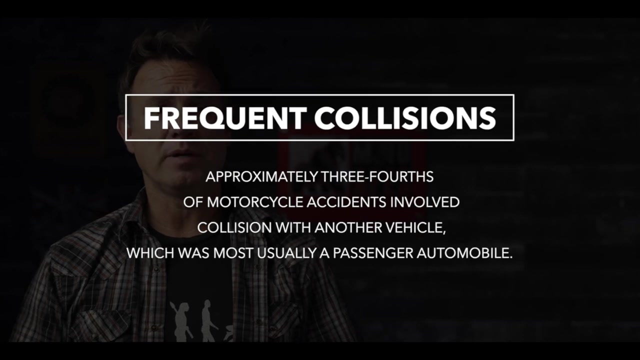 riding a motorcycle, Referencing the Hurt Report again. all the data they collected provided riders with some helpful insights to reduce our risks on the road. Here are just a few. Approximately three-fourths of motorcycle accidents involved a collision with another vehicle, which was most usually a passenger automobile. Approximately one-fourth. 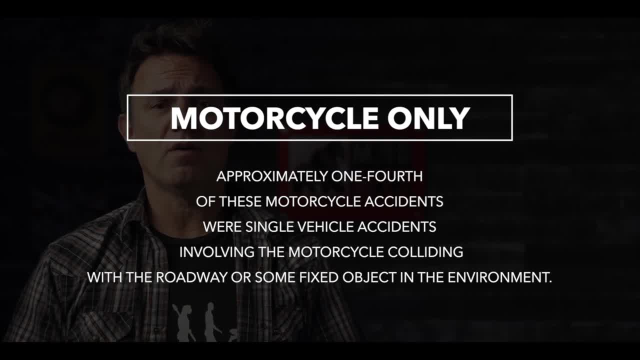 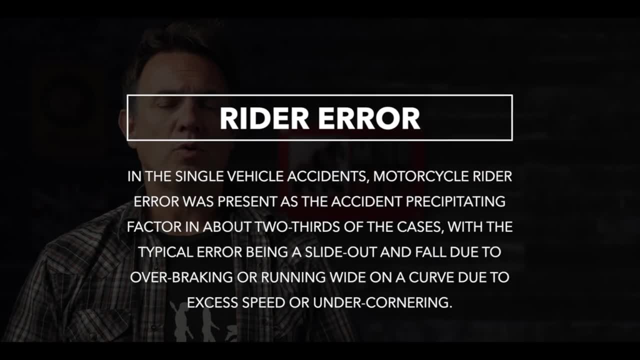 of these motorcycle accidents were single vehicle accidents involving the motorcycle colliding with the roadway or some fixed object in the environment. In the single-vehicle accidents, motorcycle rider error was present as the accident precipitating factor in about two thirds of the cases, with the typical error being a slide out. 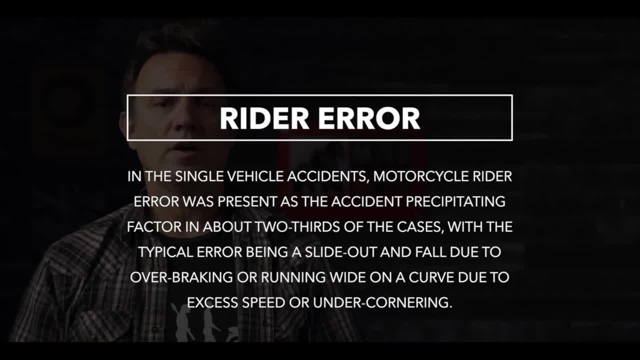 and a fall during a collision. These accidents were also shown in some wheel-to-wheel accidents with the lift off of a bike or a left-hand drive in some cases, where the weight or speed of a vehicle is due to over braking or running wide on a curve, due to excess speed or under cornering. 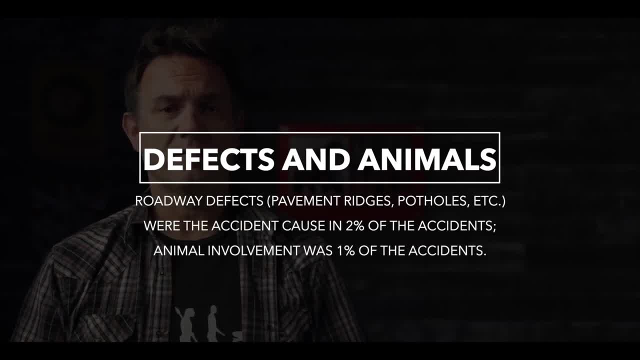 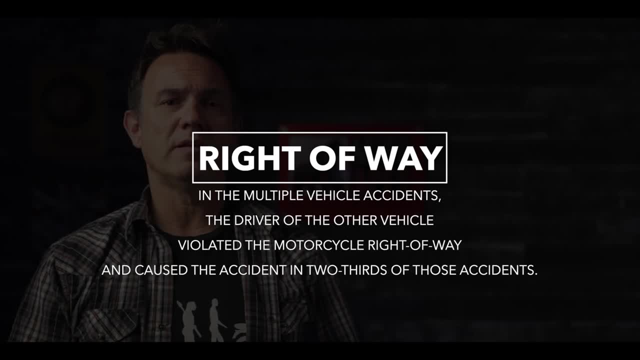 Roadway defects were the accident cause and 2% of the accidents. Animal involvement was 1% of the accidents. In the multiple vehicle accidents, the driver of the other vehicle violated the motorcycle right of way and caused the accident and two thirds of those accidents. 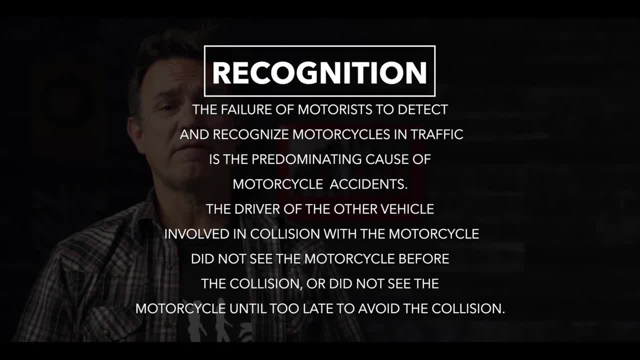 The failure of motorists to detect and recognize motorcycles in traffic is the predominating cause of motorcycle accidents. The driver of the other vehicle involved in collision with the motorcycle did not see the motorcycle before the collision, or did not see the motorcycle until it was too late. 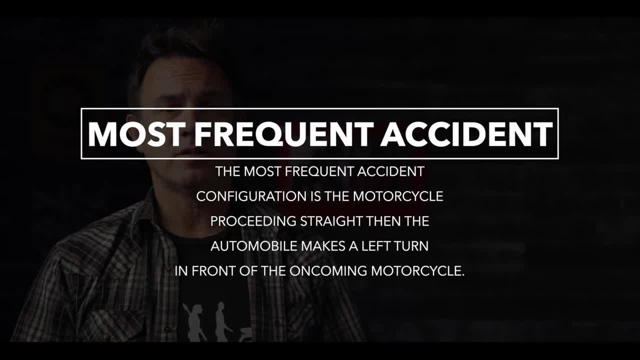 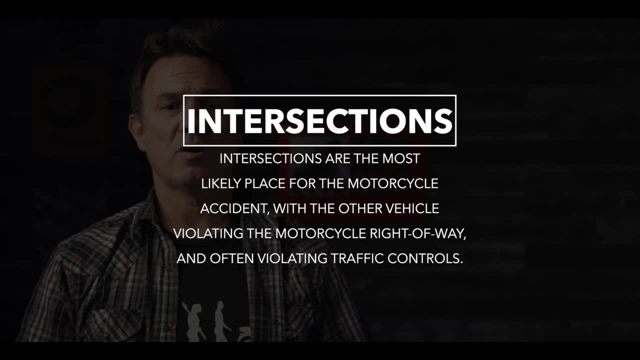 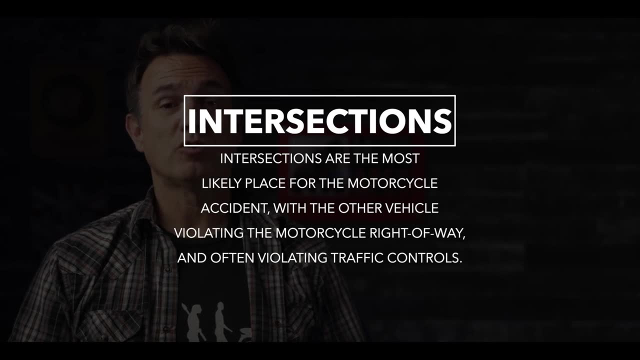 to avoid the collision. The most frequent accident configuration is the motorcycle proceeding straight. then the automobile makes a left turn in front of the oncoming motorcycle. Intersections are the most likely place for the motorcycle accident with the other vehicle, violating the motorcycle right of way and often violating traffic controls. 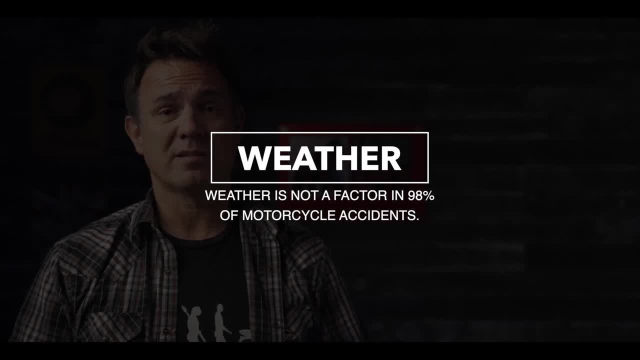 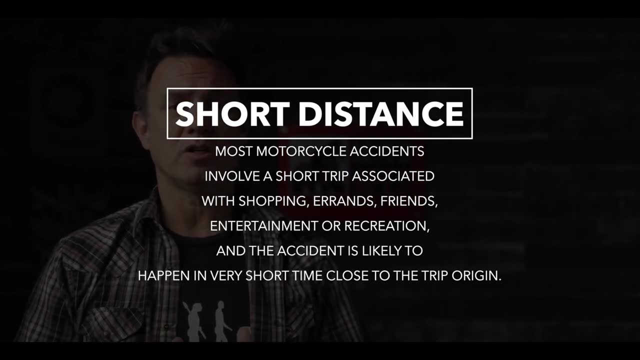 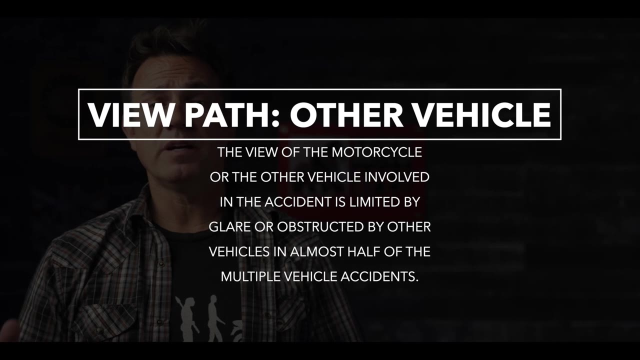 Weather is not a factor in 98%. Most motorcycle accidents involve a short trip associated with shopping, errands, friends, entertainment or recreation, and the accident is likely to happen in a very short time close to the trip origin. The view of the motorcycle or the other vehicle involved in the accident is limited by glare. 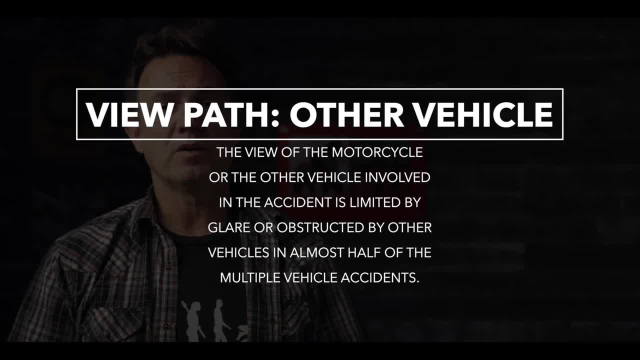 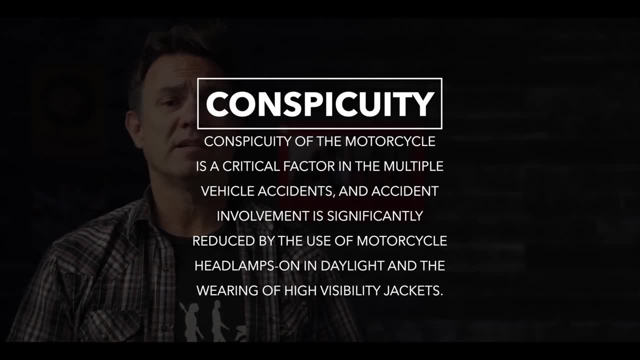 or obstructed by other vehicles and almost half of the multiple vehicle accidents. Conspicuity of the motorcycle is a critical factor in the multiple vehicle accidents. An accident involvement is significantly reduced In the winter. there are many accidents in the city. 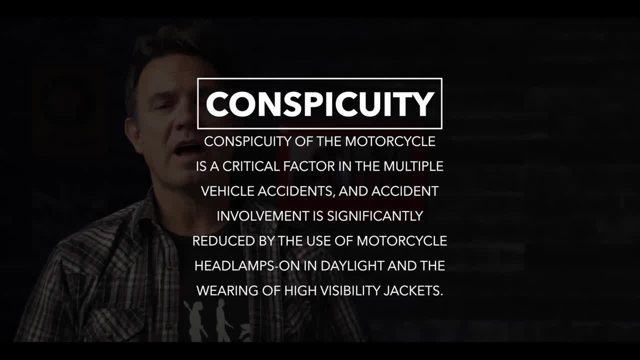 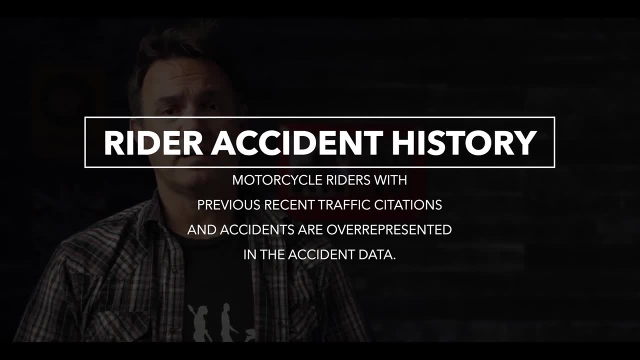 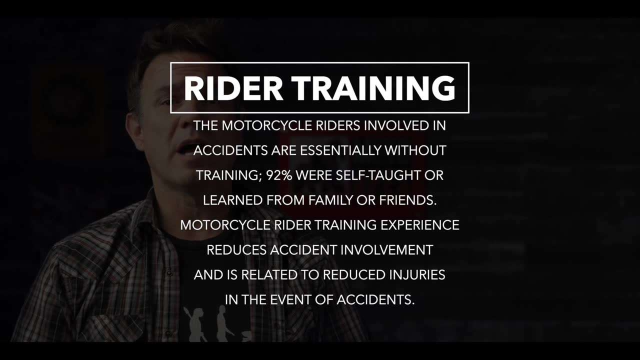 of motorcycle headlamps on in daytime and the wearing of high visibility jackets. Motorcycle riders with previous recent traffic citations and accidents are overrepresented in the accident data. The motorcycle riders involved in accidents are essentially without training: 92% were self-taught or learned from family or friends. 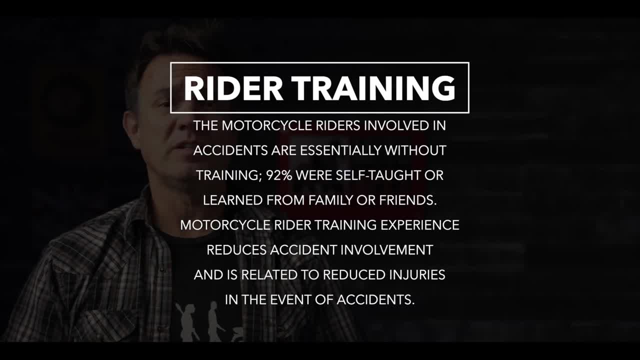 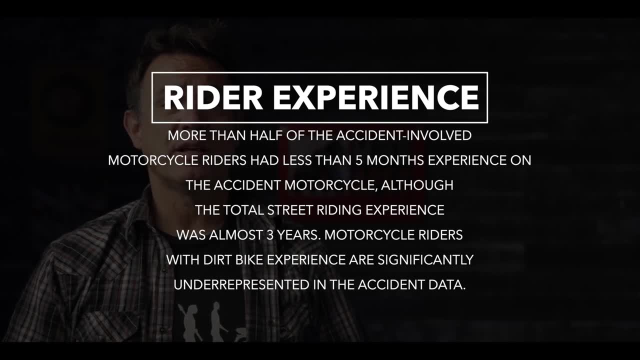 Motorcycle rider training experience reduces accident involvement and is related to reduced injuries in the event of accidents. More than half of the accident-involved motorcycle riders had less than five months' experience on the accident motorcycle, although the total street riding experience was averaged at three. 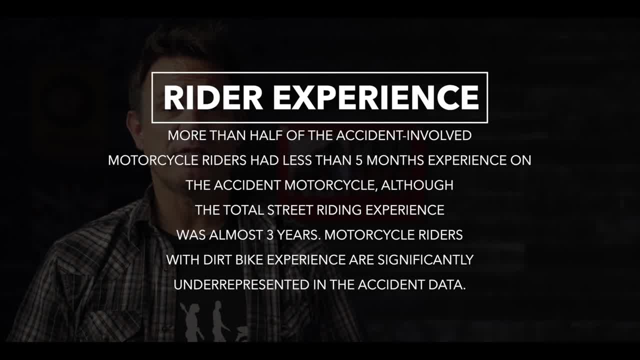 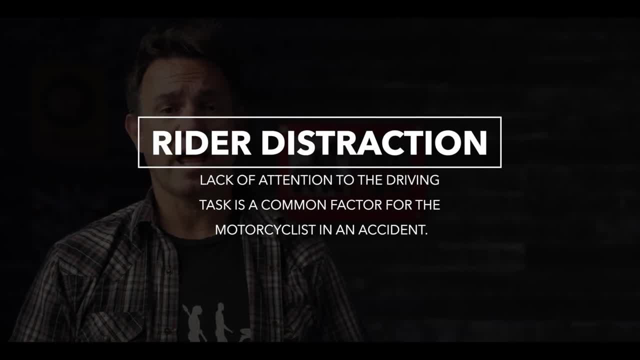 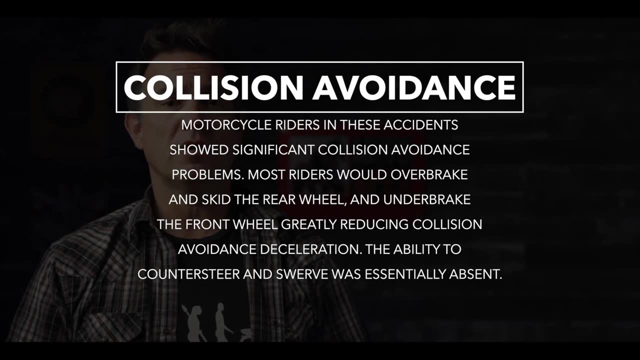 years. Motorcycle riders with dirt bike experience are significantly underrepresented in the accident data. Lack of attention to the driving task is a common factor for the motorcyclist in an accident. Almost half of the fatal accidents show alcohol involvement. Motorcycle riders in these accidents showed significant collision avoidance problems. 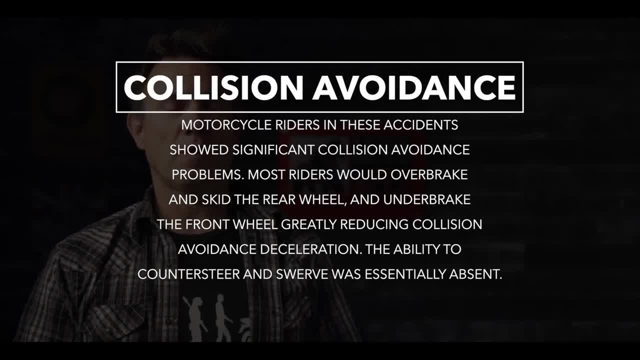 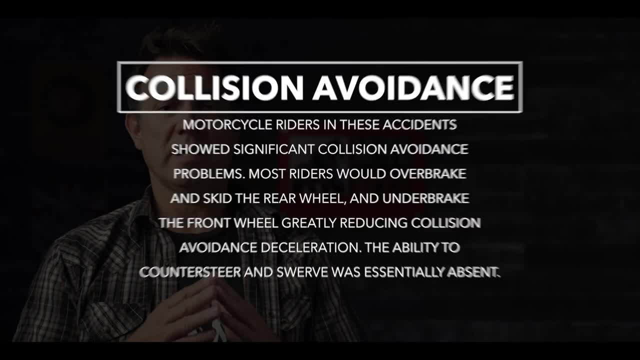 Most riders would overbrake and skid the rear wheel and underbrake the front wheel, greatly reducing collision avoidance, deceleration, The ability to countersteer and swerve was essentially absent. The typical motorcycle accident allows the motorcyclist just less than two seconds to. 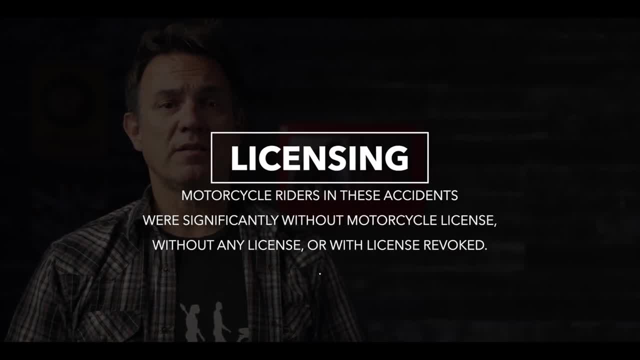 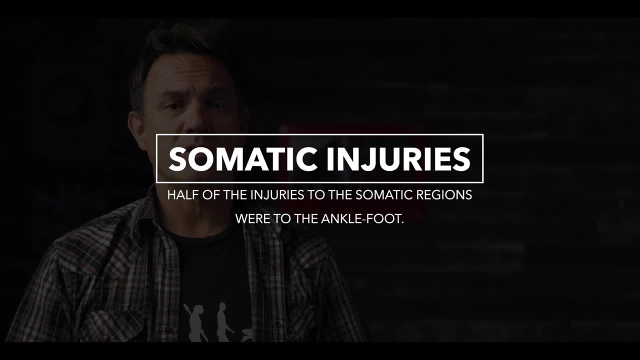 complete all collision avoidance actions. Motorcycle riders in these accidents were significantly without motorcycle license, without any license or with their license revoked. Half of the injuries to the somatic regions were to the ankle and foot. The use of heavy boots, jackets, gloves, accessories and other equipment to avoid collision avoidance. 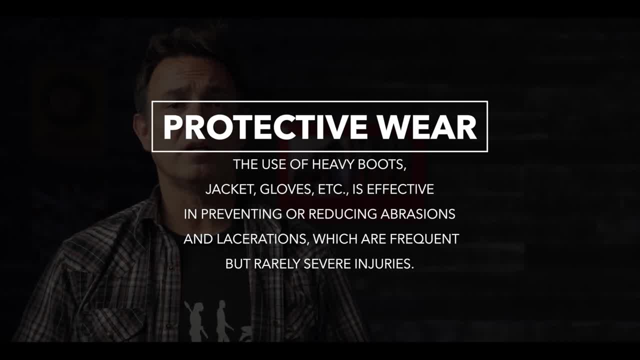 was essentially absent. Some drivers should wearist their motorcycle gloves- chocolate gloves included as well. No walkie-talkies was intensively used on pickup trucks or trams. There were chewing and skating. Most caused injuries, and injuries remainedogi cold andavorable. 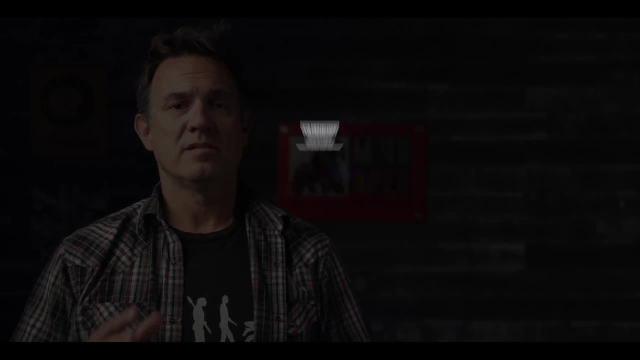 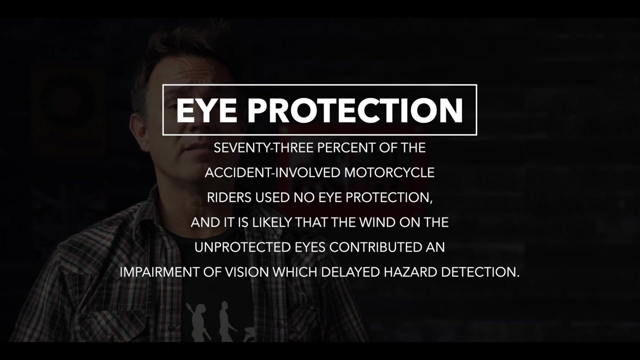 It was mostly ground Rajiva of athletes. Injury severity increases with speed, alcohol involvement and motorcycle size. Seventy-three percent of accident-involved motorcycle riders used no eye protection and most likely the wind on any unprotected eye was due to a vision impairment which delayed. 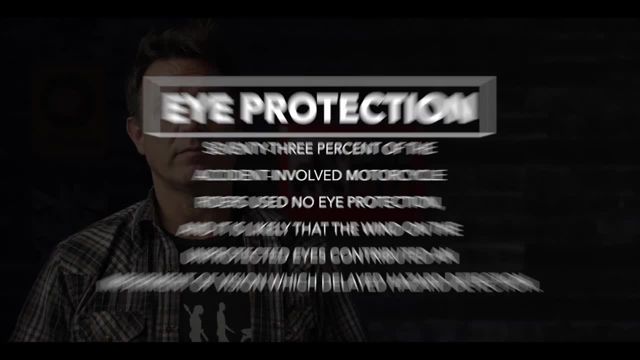 hazard detection. Severe injuries also drawedкие injuries was known to increase death and financial aid on the motorcycle knew developing motorbike users in a particular vehicle would be necessary pour through city. JUST NOTE Noting that safety helmets werelatest for untrained. 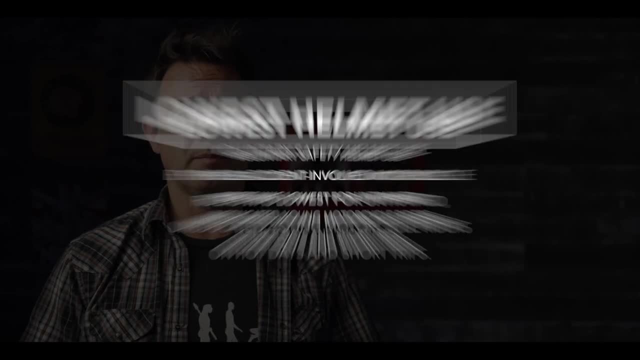 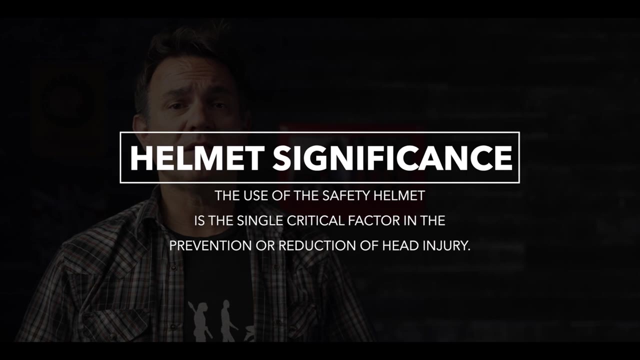 uneducated young motorcycle cyclists. canопies and comet Sanskrit, trim, Kobe, are and Wirtschafts are on hot days and on short trips. The most deadly injuries to the accident victims were injuries to the chest and to the head. The use of the safety helmet is the single critical factor in the 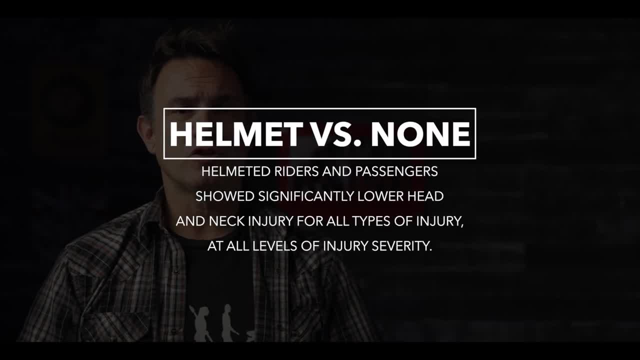 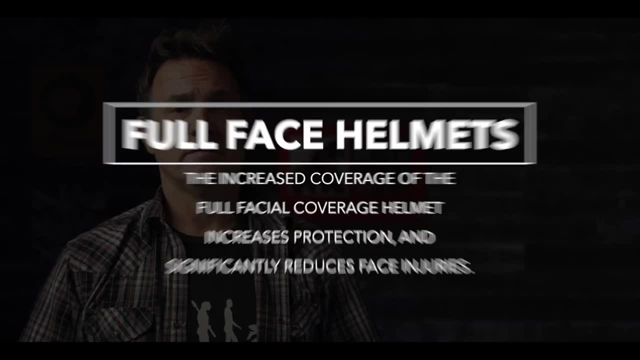 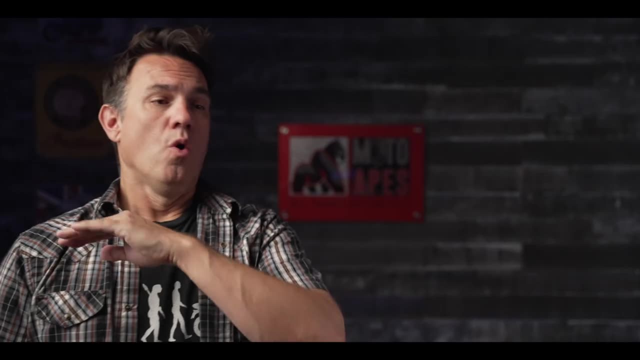 prevention or reduction of head injury. Helmeted riders and passengers showed significantly lower head and neck injury for all types of injury at all levels of injury severity. The increased coverage of the full facial coverage helmet increases protection and significantly reduces facial injury. So back to the topic: how safe are motorcycles? If you've been listening to all the 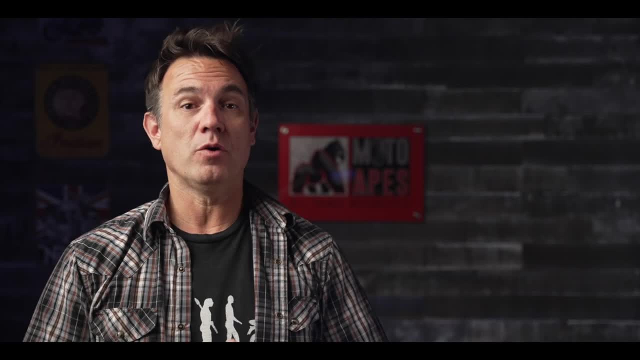 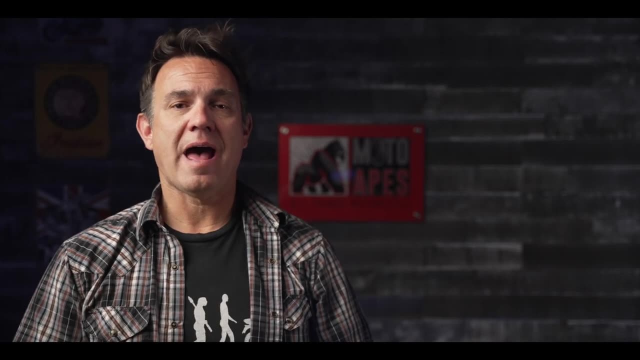 doom and gloom here. you might agree with that friend or family member warning you and conclude: not very. Perhaps a better question is: how safe of a rider am? I Sure accidents are going to happen. That's why they're called accidents. But combing through the data and it's very clear the rider's 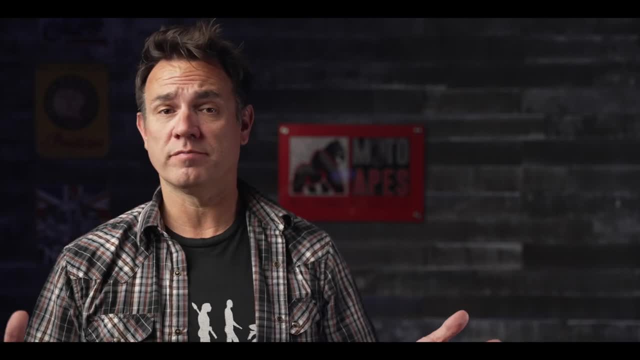 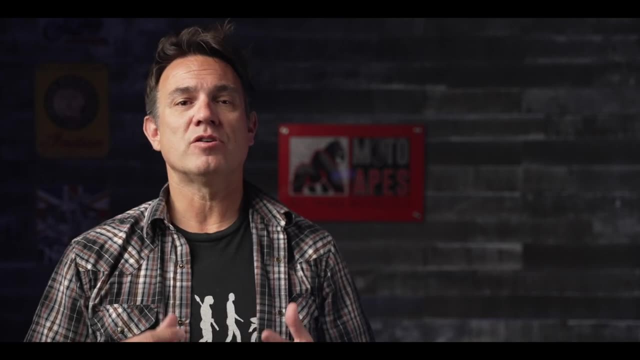 role in protecting him or herself from injury or worse. Mitigation is everything. When 98% of all motorcycle accidents result in an injury: the rider's role in protecting himself or herself from an injury of some type. the best thing we, as riders, can do is everything we can to avoid. 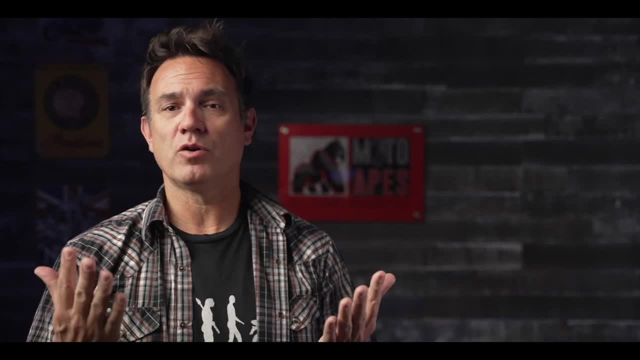 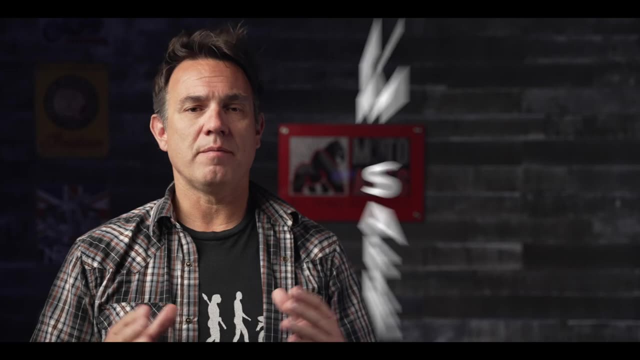 accidents in the first place. I'm a professional pilot and maybe the motorcycle community could learn some things from what is considered to be the safest form of transportation in the world. Pilots use the I'm safe checklist. It's an acronym taught early on in flight training and it's used 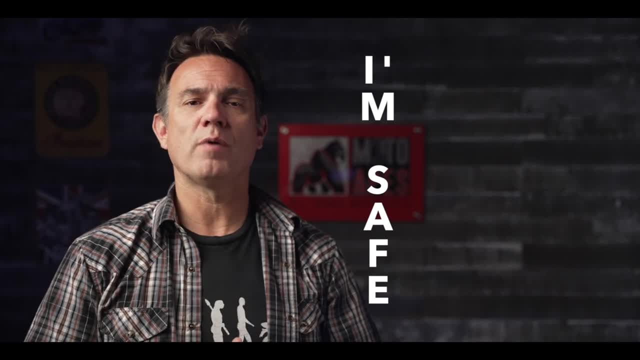 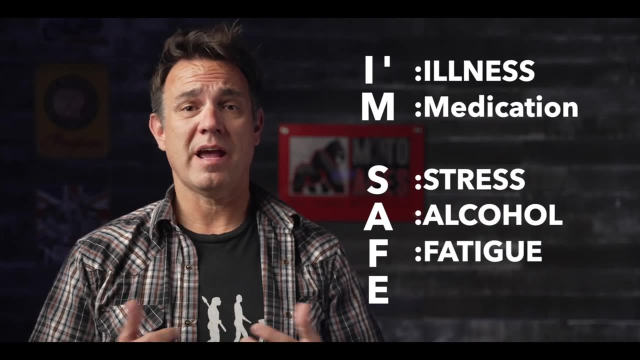 throughout a pilot's professional career to assess their overall readiness for flight when it comes to illness, medication, stress, alcohol, fatigue and health. So if you're a pilot and you're a professional, you can also identify yourself as a pilot and take these actions into account. 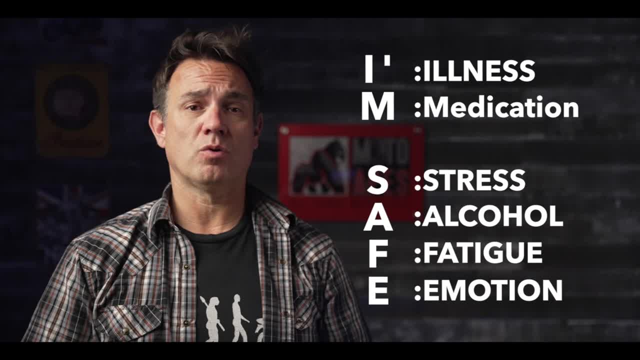 For example, if you're a pilot, you need to be clear about your safety standards. You can also be clear about your safety standards when you're on the road, when you're on the highway, when you're on a red flag. all of these can have a negative impact on a rider's ability to maintain safe. 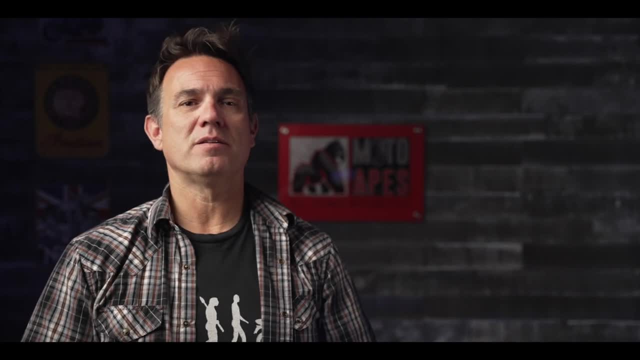 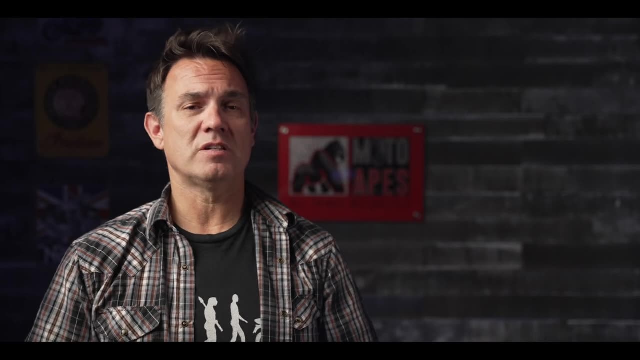 effective control of their bikes. Another thing pilots must address is hazardous attitudes. I've witnessed many new riders, especially young ones, with complete disregard to the safety risks associated with riding a motorcycle And, more times than not, older, more experienced riders who 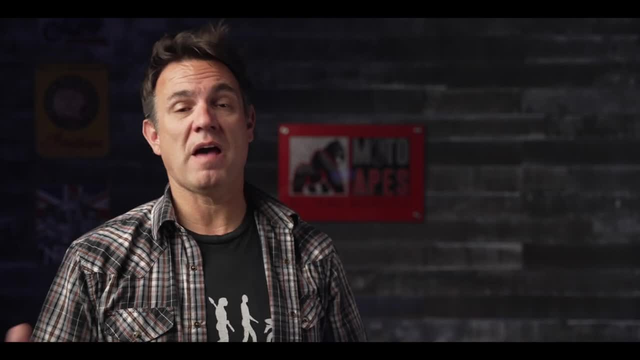 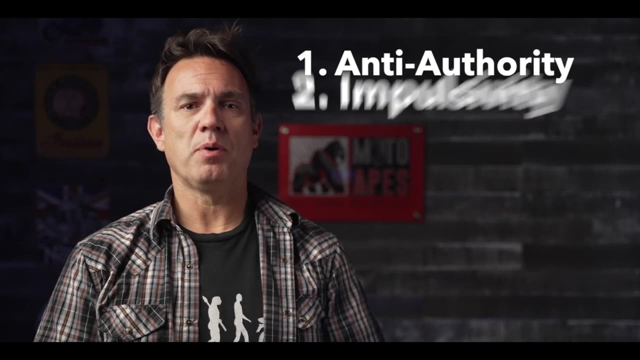 lost respect for the dangers of motorcycle riding, just becoming complacent or developing an unsafe attitude. Before you ride, be mindful of the dangers of five hazardous attitudes like anti-authority, impulsivity, invulnerability, machoism, resignation. Pilots are trained to be. 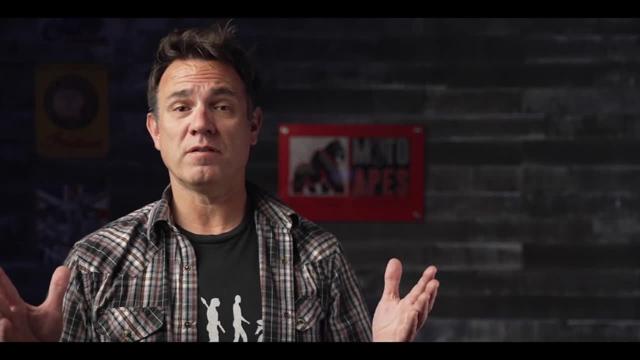 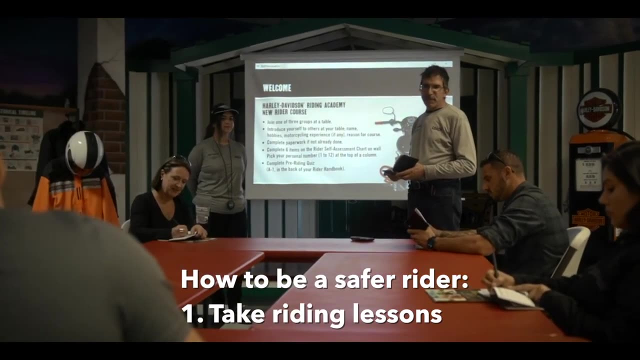 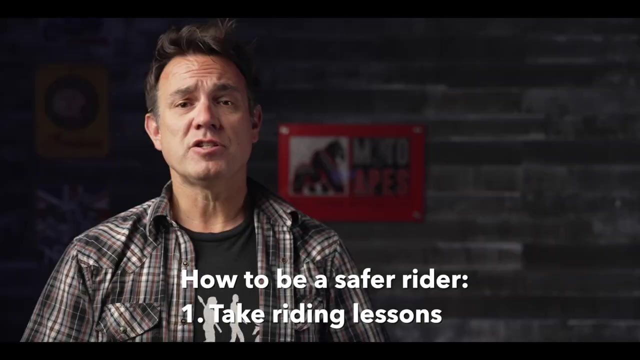 safe They go to school. Want to make your motorcycle safer? Be a safer rider. How do I make myself a safer rider? One take lessons. The Motorcycle Safety Foundation has basic rider courses and continuing education courses for more advanced riders. Educated riders are proven to be. 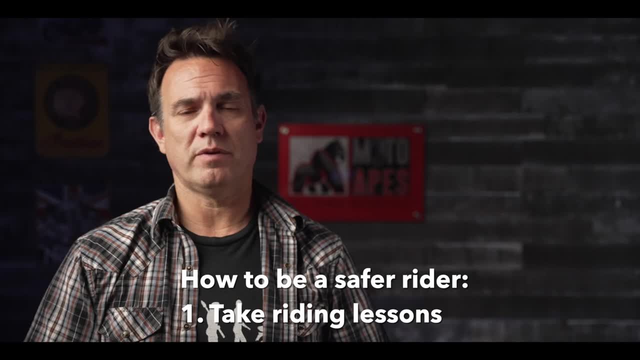 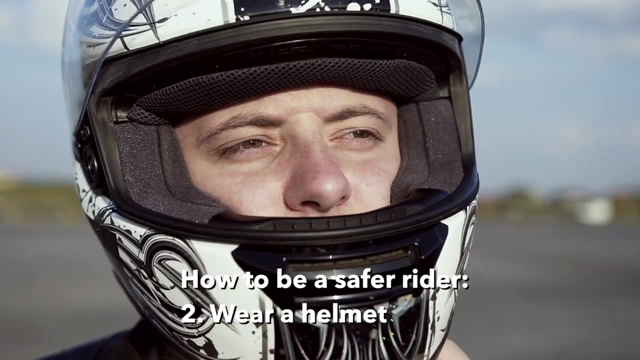 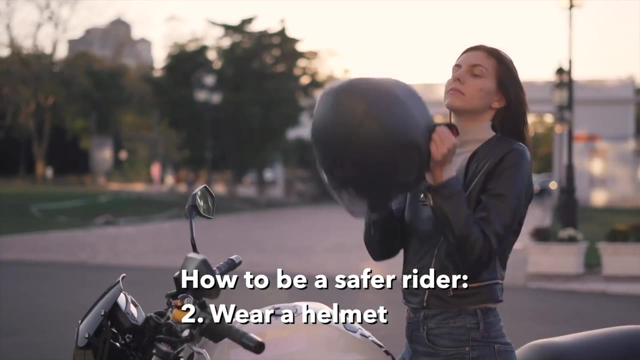 safer riders. so keep learning. There is no pinnacle you can reach. Get better and get safer. Number two: wear a helmet. Just because it's not the law in your state doesn't mean it hasn't been proven to save lives. Additionally, wear a full face helmet. This has been proven to save riders. 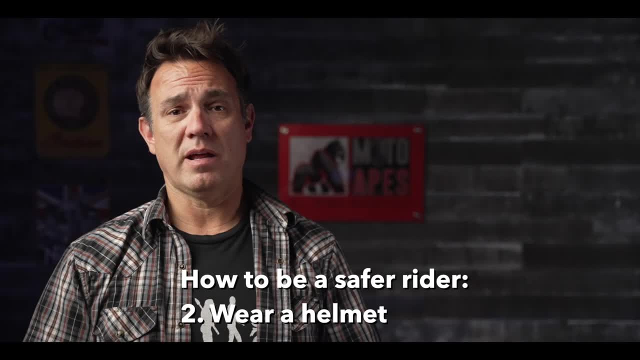 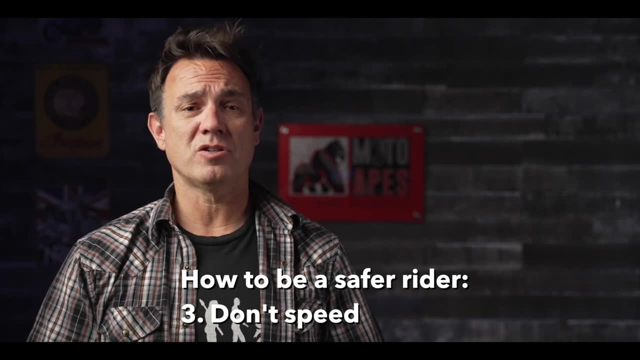 from serious face and eye injury. Number three: don't speed. Not only does speed help you save lives, but it also helps you save lives. So don't speed, Don't speed Increase the chance of you losing control and being involved in a single vehicle crash. 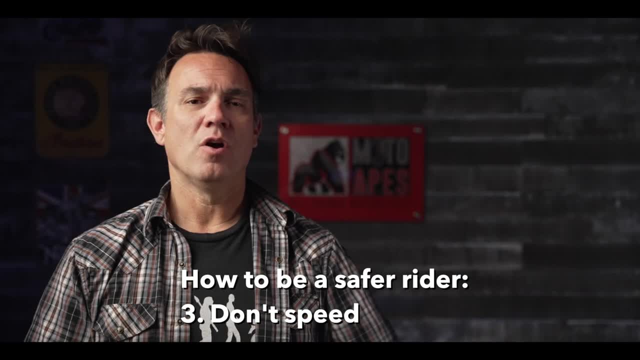 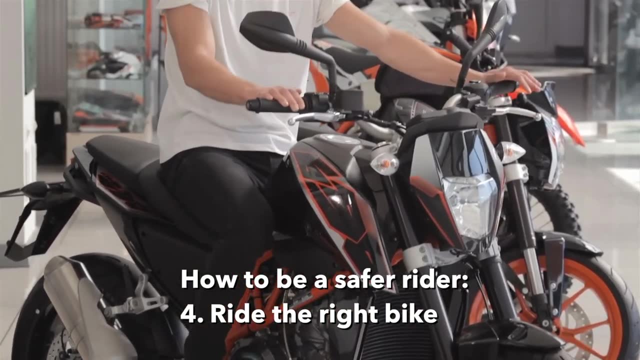 It also reduces your reaction time for that inevitable time where a car makes that left turn in front of you. Number four: ride a bike appropriate to your skill level. Don't jump on a super sport as your first bike because you thought it looked cool when someone was doing. 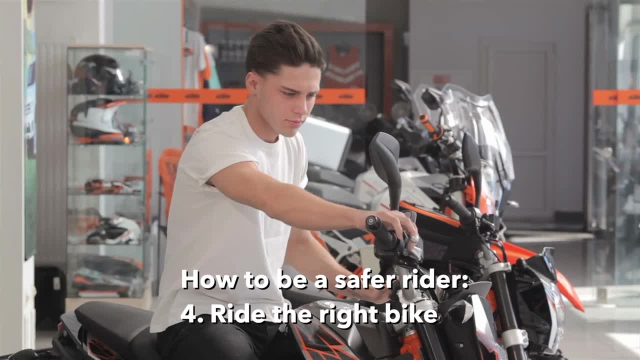 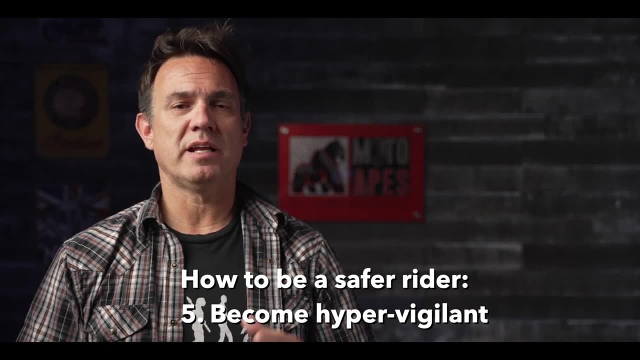 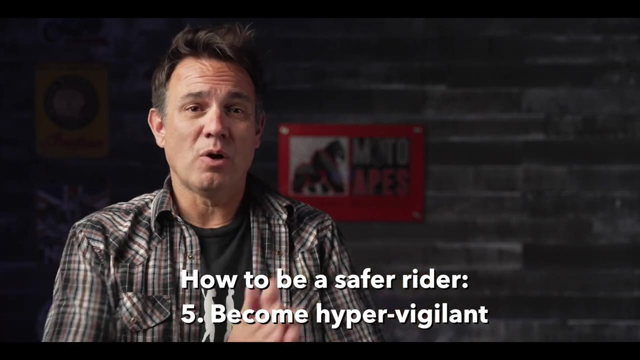 wheelies on one down the freeway. Younger riders with no experience- we're talking to you. Number five: become hypervigilant. Pay attention, especially when approaching an intersection. If you know that most fatal accidents occur at intersections, pay attention. dude, Approach, slow. 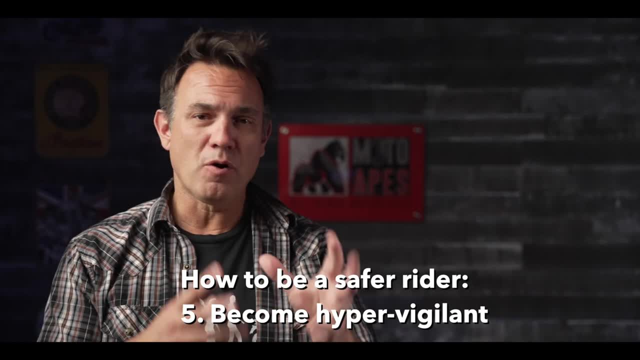 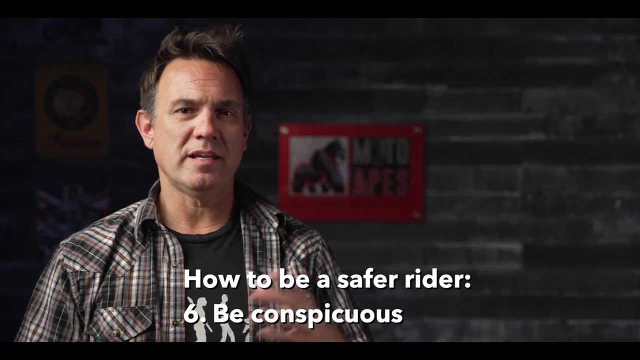 Expect the worst and be prepared. I know we all like our Ram smartphone mounts, but keep your eyes forward, especially in the city. Number six: be conspicuous: Bright, yellow, white, high visibility clothing, daytime running lights, car drivers who've hit motorcyclists. 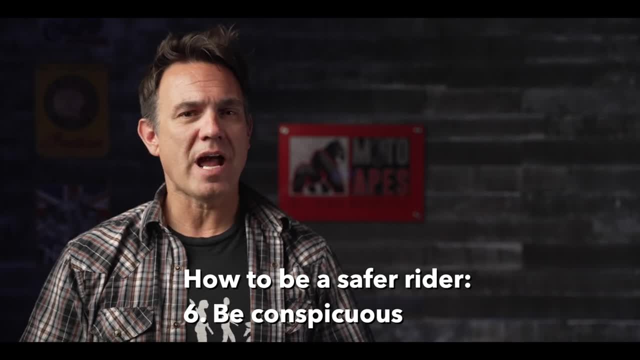 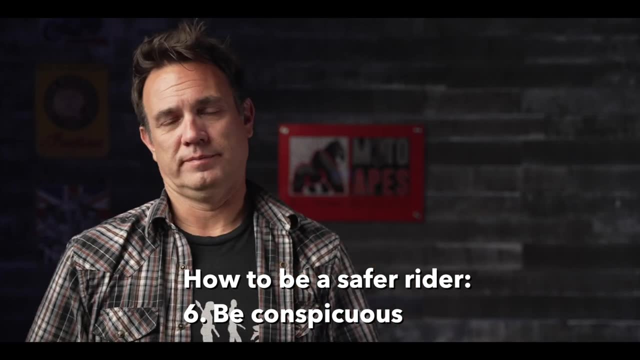 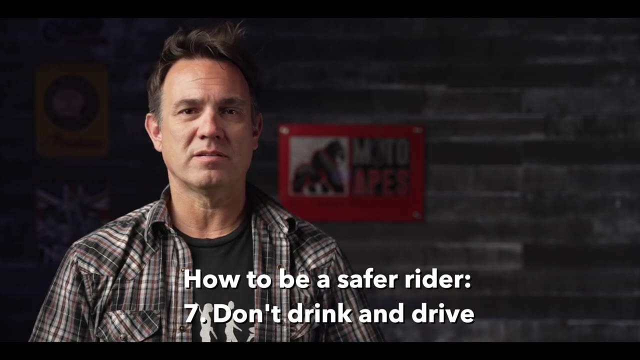 said they couldn't see them or didn't notice. I know that black leather jacket is cool, but it's not that cool. Put on a safety vest if you have to, but let the cagers know where you are. Number seven: don't drink and drive, Just don't. A totally unworth it and unnecessary risk If you. 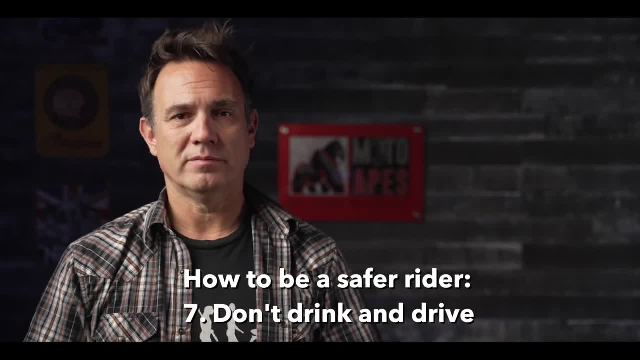 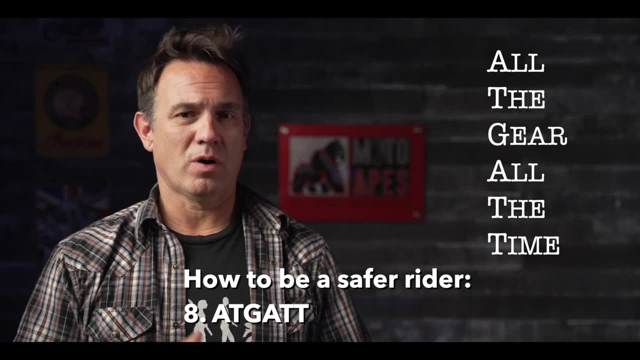 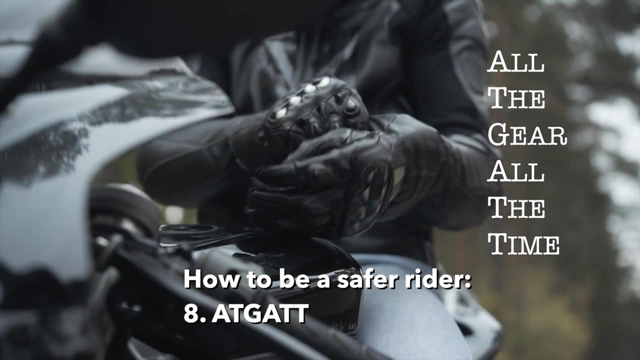 do catch an Uber home, live to ride another day. Number eight at-gat, All the gear all the time. Just because an accident won't kill you doesn't mean it won't hurt. When most accidents occur shortly after a ride begins from home and on errands, protect yourself, especially your hands. 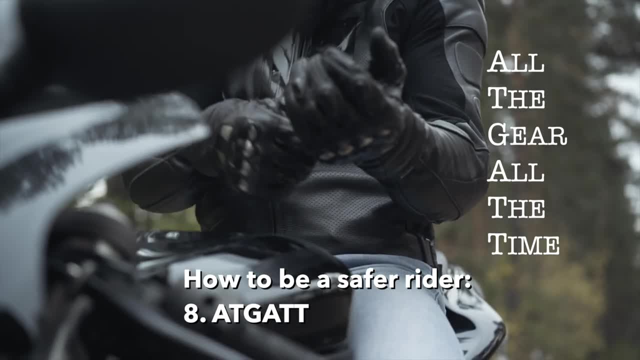 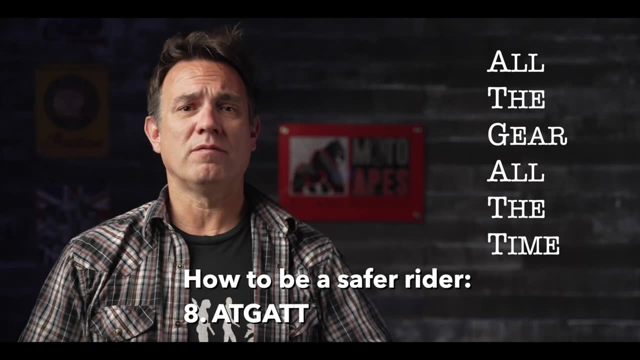 Your knees, your feet, your chest, your head, your whole body, If you like, your skin. ride with CE-rated pants and jackets. Wear boots, High boots, because there are an overrepresented amount of leg injuries to the tibia and fibula, Armed with the information about the greater risk of fatality due to rib. 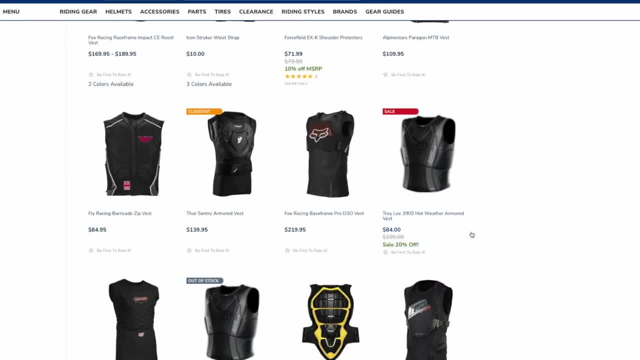 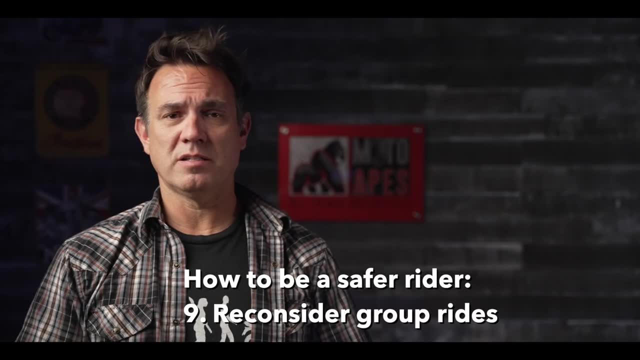 fracture and thoracic injury. it's time also to seriously consider the use of chest protectors all the time as part of our at-gat kit. Number nine: avoid group rides with inexperienced riders and people you don't know. More times than not, you're going to have to be careful If you're not. going to be able to ride, you're going to have to be careful. If you're not going to be able to ride, you're going to have to be careful. If you're not going to be able to ride, you're going to have to be careful. 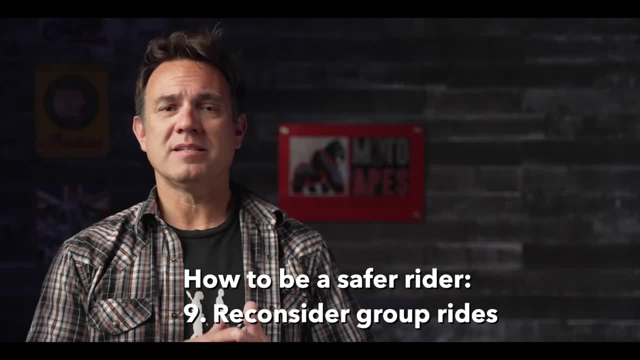 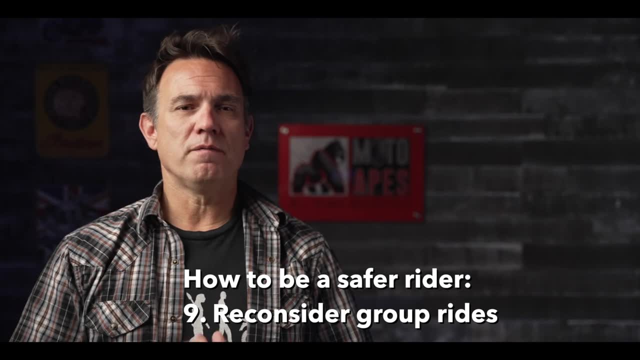 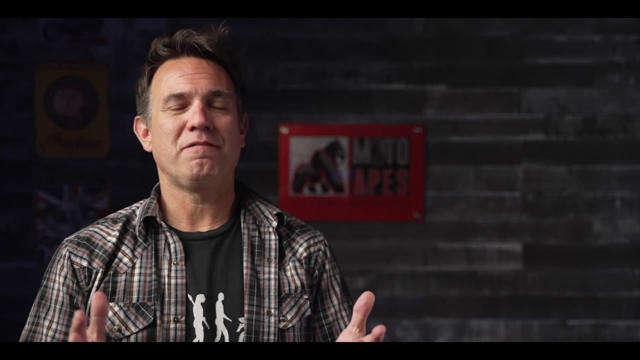 More times than not, group rides lead to accidents because inexperienced riders can't hold their lines. Hell, it could even be you. If you must ride in a group, make sure you've thoroughly briefed your route and expectations with your fellow riders. So, in closing, how safe.